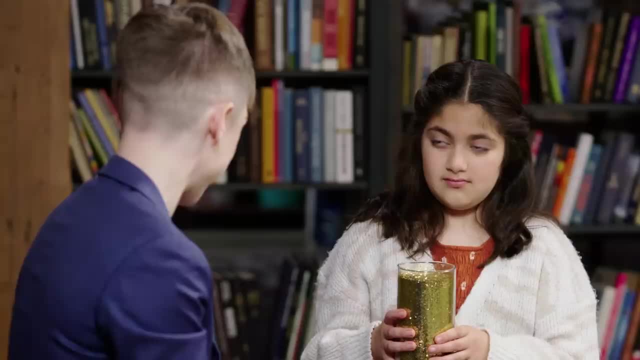 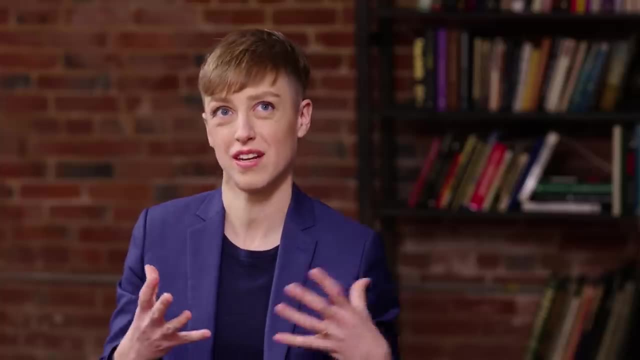 An infinite amount of jars, Very good. Why do you say that? Because if there's unlimited pieces of glitter, we need unlimited pieces of jar. So let's try and imagine infinitely many jars. Would they fit in this room? Yeah, No. 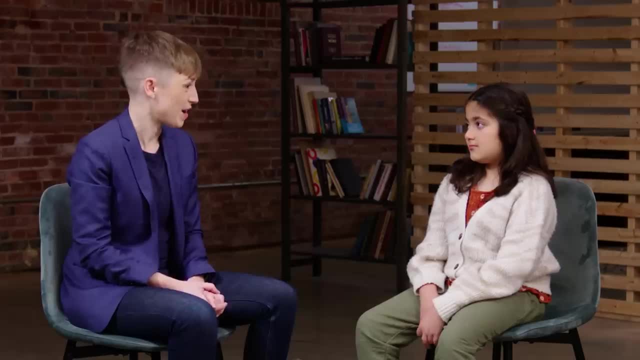 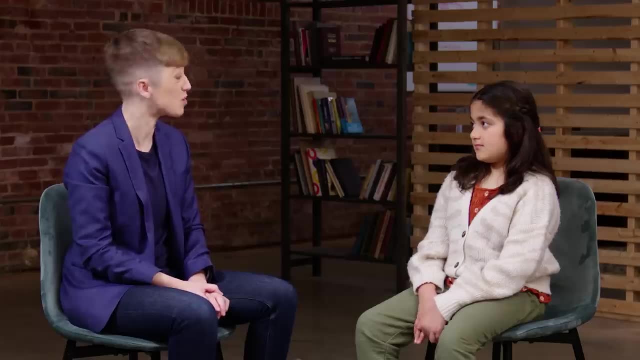 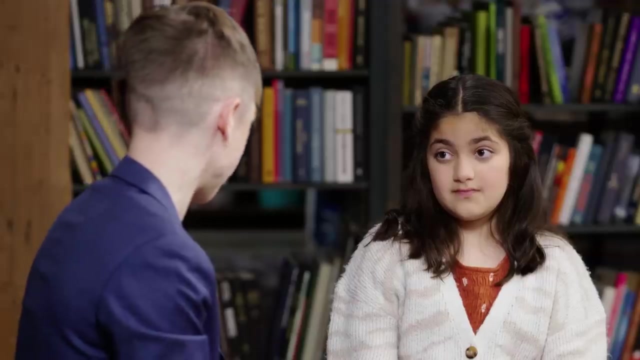 Yeah, absolutely not, because this room holds only a finite amount. A finite amount of space And, in fact, infinitely many jars would not even fit in something called the observable universe, which is the portion of the universe that astronomers can see. How does that make you feel? 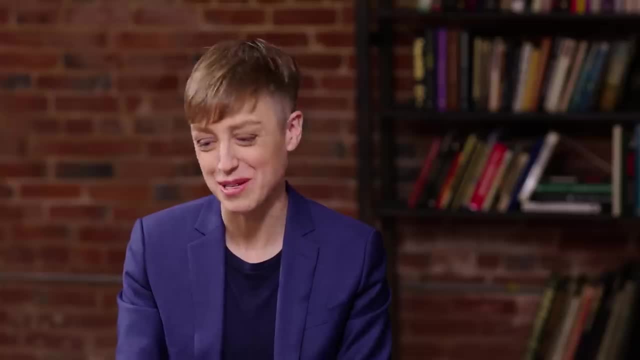 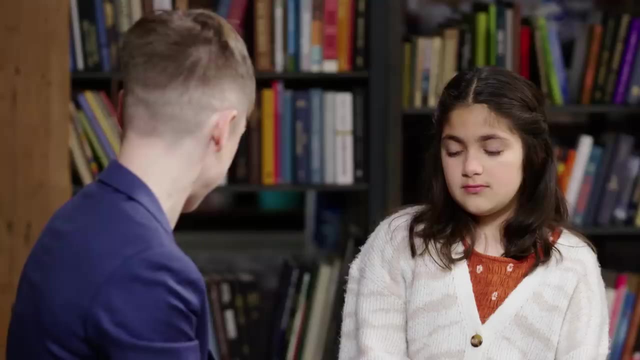 That makes me feel like my brain is exploding? Yeah, that makes me feel like my brain is exploding. Can infinity ever get bigger? That's a wonderful question, a very rich question. What do you think? I think maybe because you said it was unlimited. 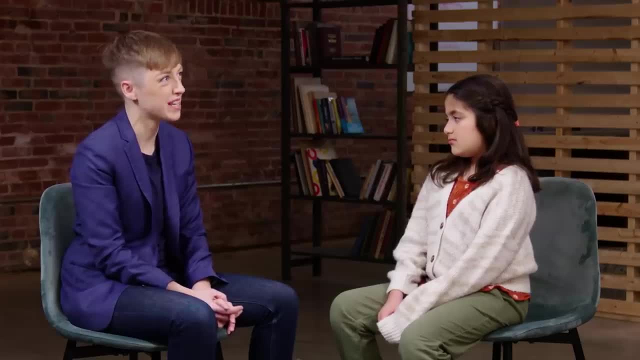 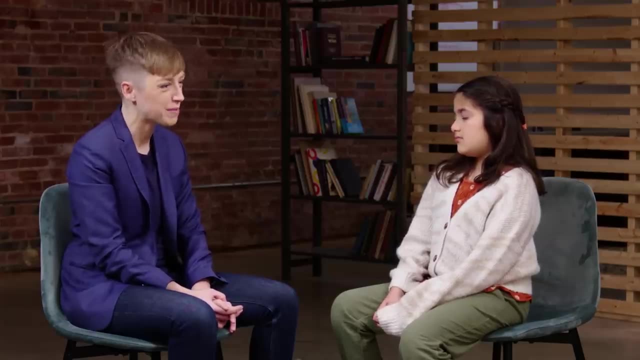 It's a very good intuition. So there are ways that mathematicians can build infinite collections of things, and if you repeat those processes, it's in fact possible to build even bigger and bigger sizes of infinity. So what have you learned today about infinity? 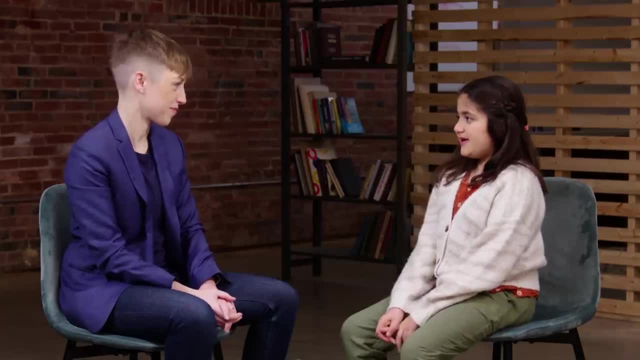 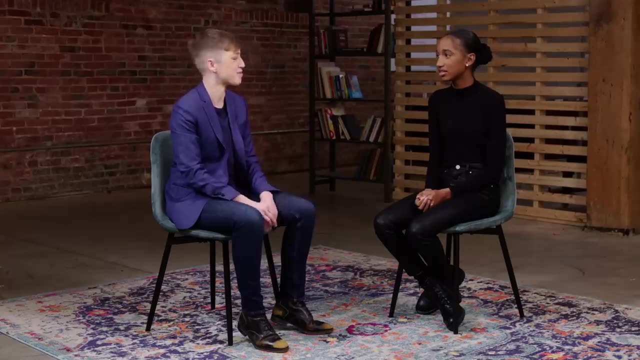 I've learned that, even if it's unlimited, there are many different ways of making infinity, and you can never actually see it all. What does infinity mean to you? It means anything that has no end to it. Yeah, that's absolutely right. 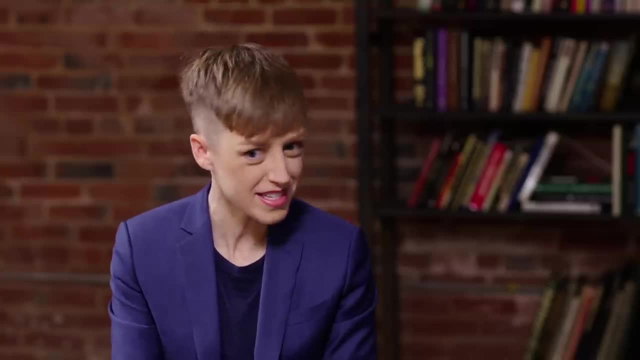 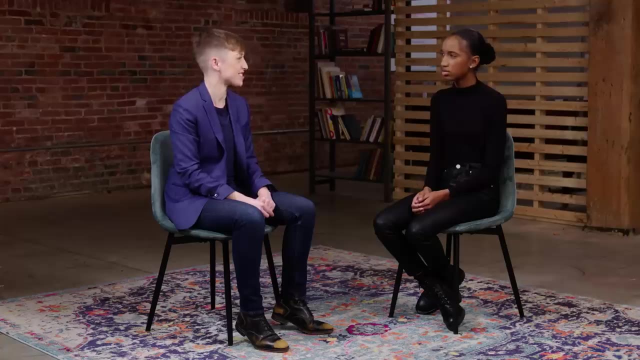 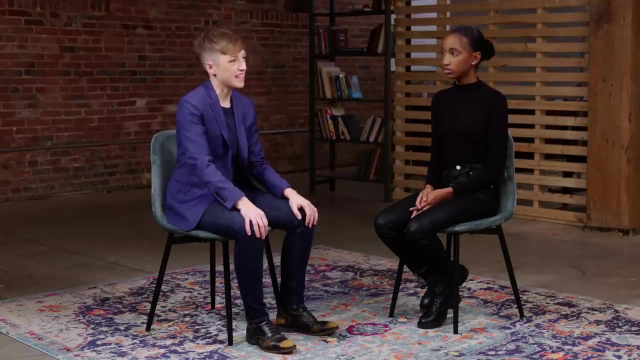 So infinity gets used a lot of different ways in mathematics. There's a way that mathematicians think of infinity as a number, just like the number 13,, just like the number 10 million. Wow, okay. So the reason that mathematicians consider infinity to be a number is that it is a size of a set. 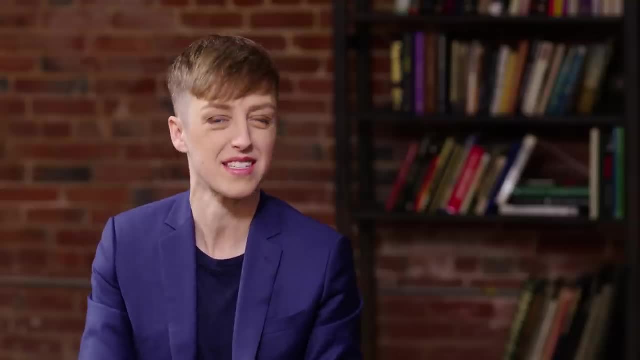 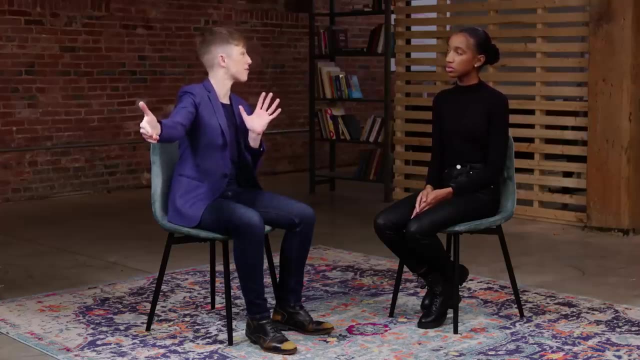 So the first example of an infinite set in mathematics is the set of all counting numbers, So one, two, three, four, five, six, seven. That list goes on forever. That is an infinite set And to be a little bit more precise, it's a countably infinite set. 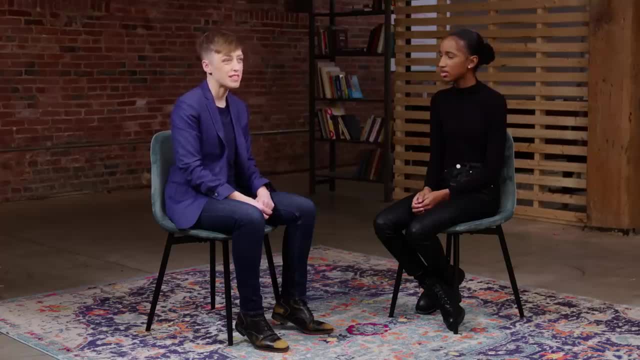 But as a number, infinity is pretty strange. What do you mean by that? Adding infinities, multiplying infinities, And there's a sense in which it's very similar to the arithmetic that you learned about already, but it's also totally different. 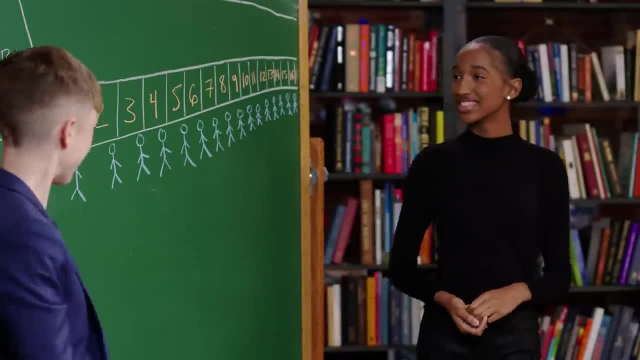 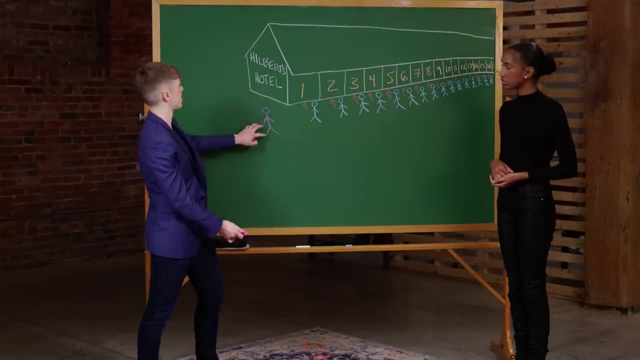 It has some very weird properties. Welcome to Hilbert's Hotel. Unlike an ordinary hotel, it has countably, infinitely many rooms. Suppose a new guest shows up, You might think that the new guest could take the room that's all the way down at the end of the hall. 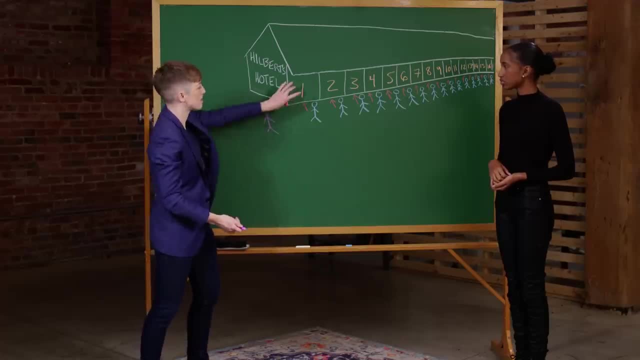 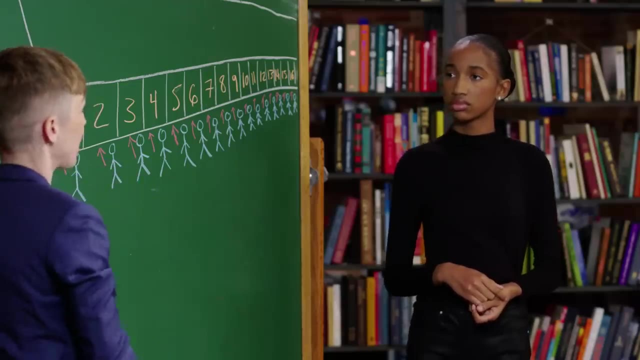 all the way at infinity, Except there isn't a room like that. The rooms each have a number, And even though there's infinitely many rooms, each room is only a finite distance away. So here's how we're going to make room for the new guest. 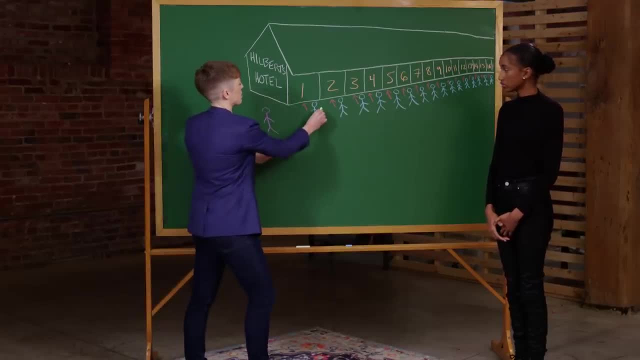 I'm going to ask the guest in room one to move into room two, And then we're going to ask the guest in room two to move into room three, And we'll continue this all the way along. It looks to me like there's space for the new guest. 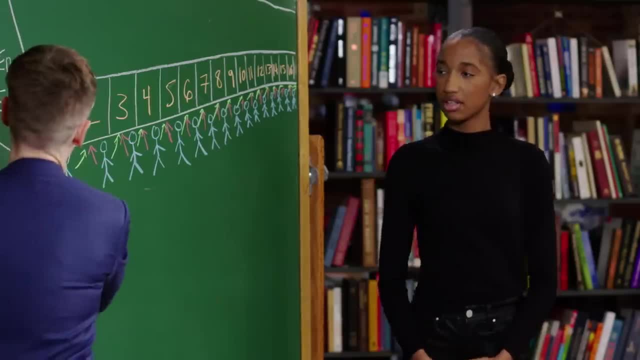 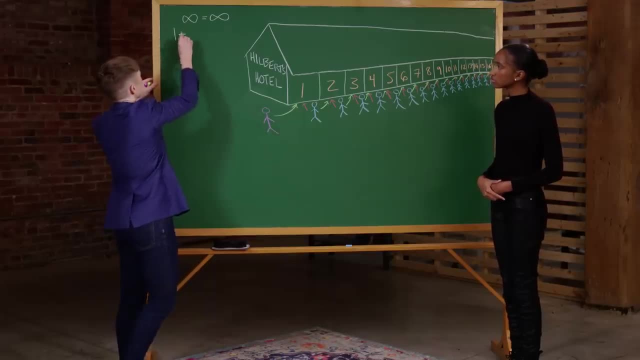 Where is it? It'll be in room number one, Room number one Exactly. I'm going to use this symbol for infinity, But what we've just shown is that one- the one new guest plus infinity is equal to the same infinity. 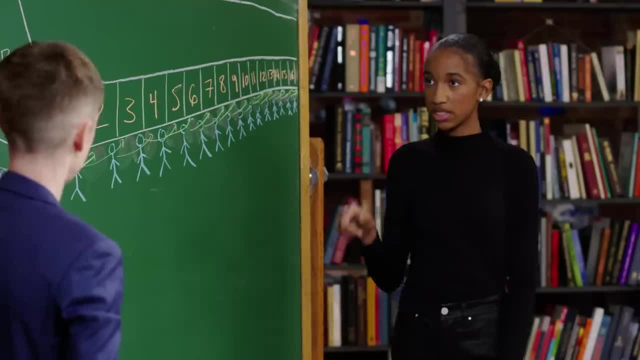 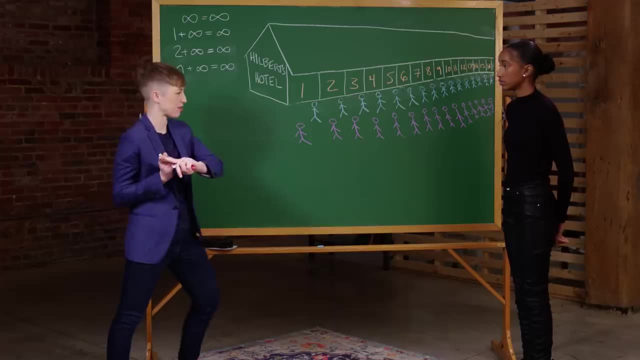 What happens if we had a second guest? Would it be? two plus infinity equals infinity, Absolutely Okay. So now I'm going to make this story a little more complex. There's another Hilbert's hotel down the street And they're having plumbing issues. 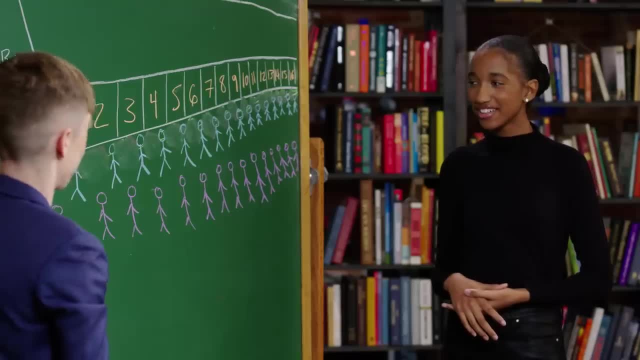 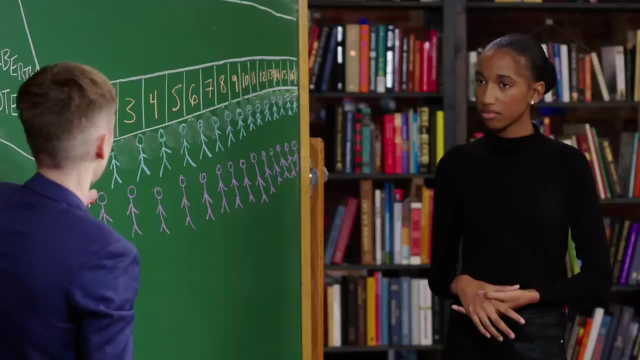 And we need to find room for them. Okay, They can't live together. They can't live together. That would be a great solution. I don't know. I think these people don't really get along, So I need to somehow create infinitely many new rooms. 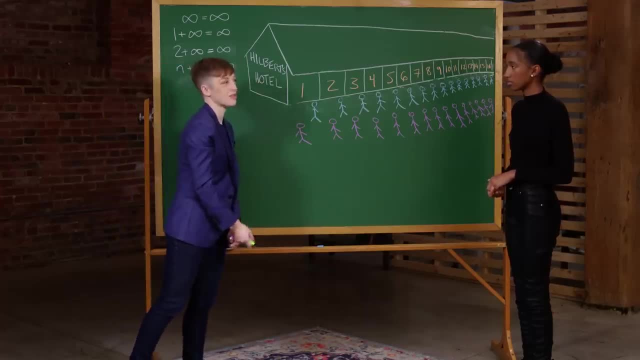 But I can only ask each person in the hotel to move a finite distance away, Right, So let's take the guest who was originally in room one And move them into room two, So that's creating one new space for us, And I'm going to take the guest who was originally in room two. 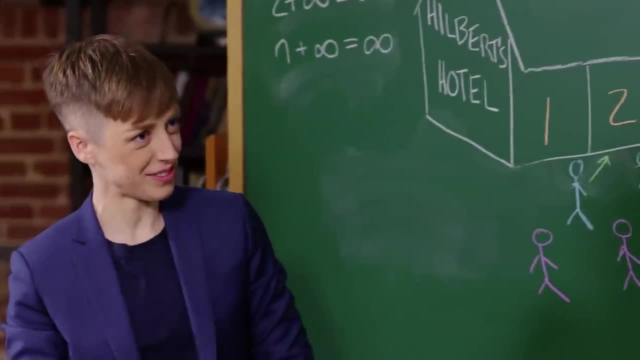 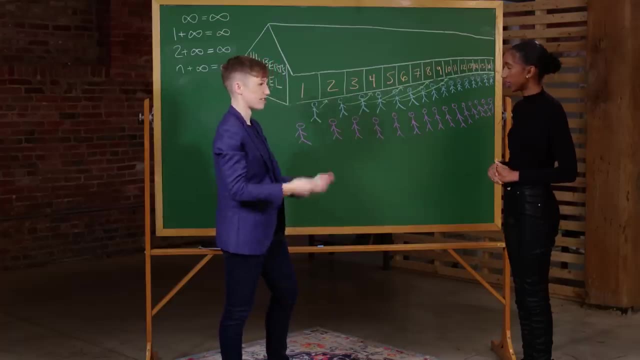 And move them into room. four: Are you starting to see a pattern here? Yes, You're going up one each time. Yeah, I'm increasing by one more each time, So I'm doubling the room number, in fact. Right, So this is some of the strange arithmetic of infinity. 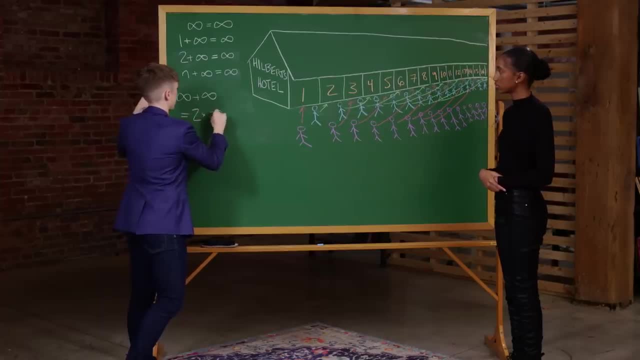 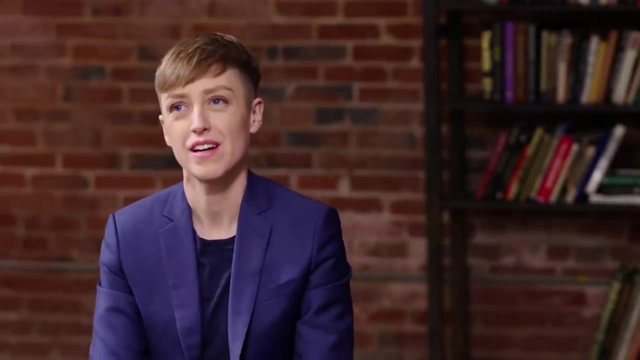 So we have two Hilbert hotels, Each of which have infinitely many guests. Right, Which is equal to Infinity. Infinity Great Hilbert's Hotel is a story that mathematicians have been telling themselves for almost 100 years, Because it's a really visceral way to think about some of the counterintuitive properties. 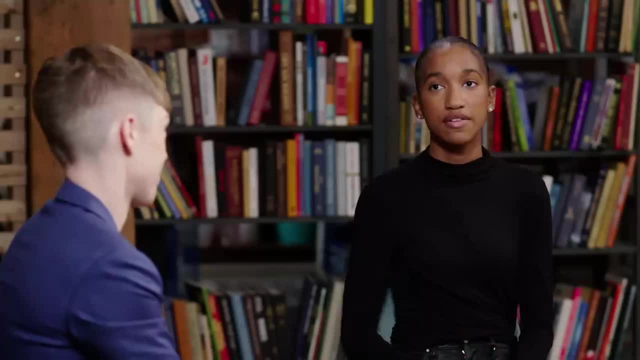 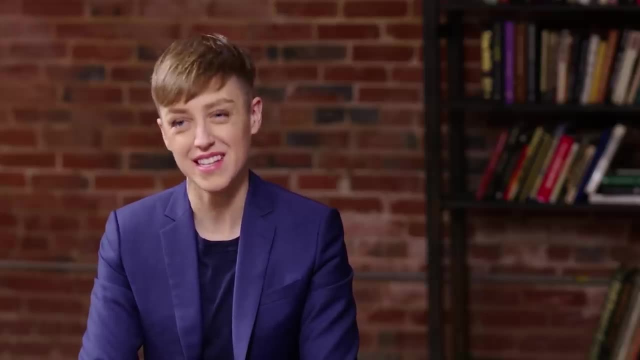 of the arithmetic of infinity. How does infinity come across in mathematics for you? So when I'm teaching calculus and talking about concepts like limits and derivatives, those are only defined precisely with infinity, Mm-hmm. When I'm teaching algebra, which is meant in a different sense, about number systems, 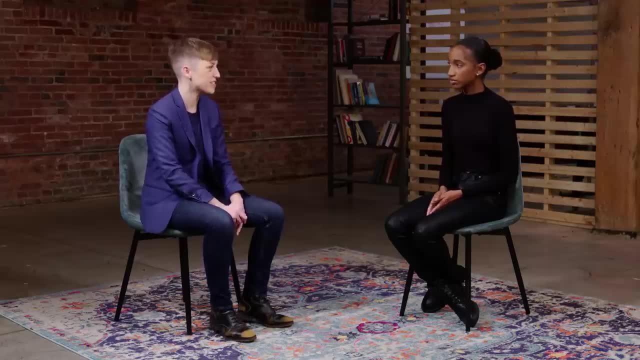 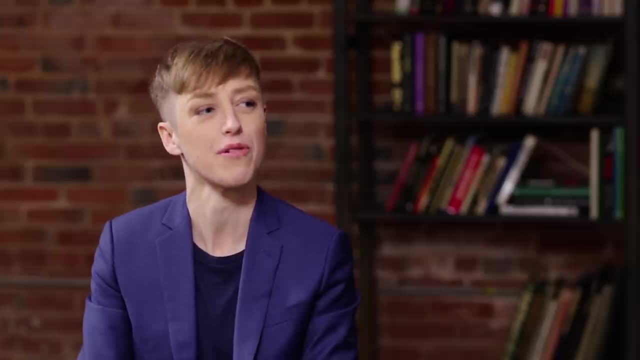 we deal with infinite families of numbers and their operations, Right, Mm-hmm? Infinite sets are somehow very exotic, Mm-hmm. They're not found so commonly in the real world, but they're all over mathematics, Mm-hmm. 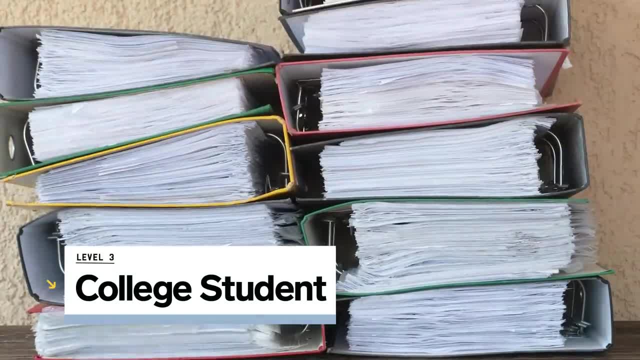 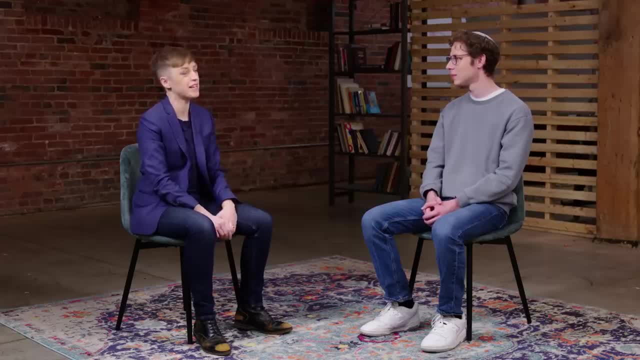 Mm-hmm. What do you know about infinity, The property of something being endless Great. So today we're going to focus on infinity as a cardinality. And what cardinality means is it's a size, Right. What cardinality means is it's a size of a set. 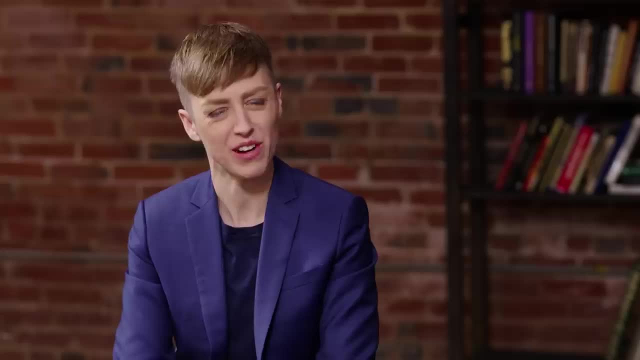 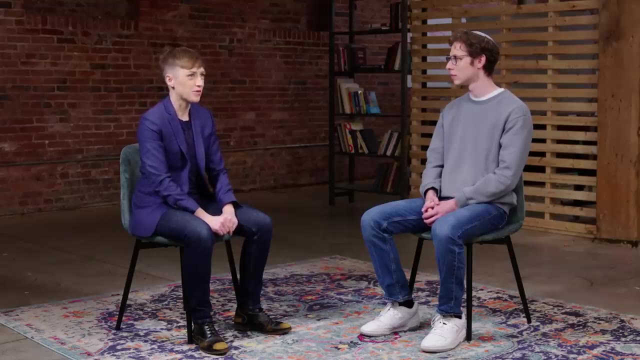 What are you studying? I'm studying computer science. Studying computer science: Mm-hmm. Are you taking any math courses right now? Yeah, Right now I'm taking calculus 2.. Calculus involves the study of functions. Functions are one of the most fundamental concepts in mathematics, but they aren't always. 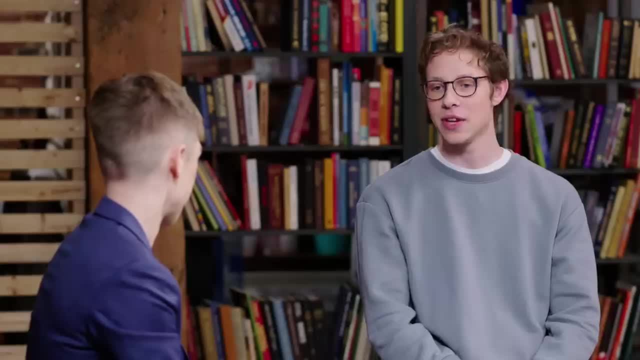 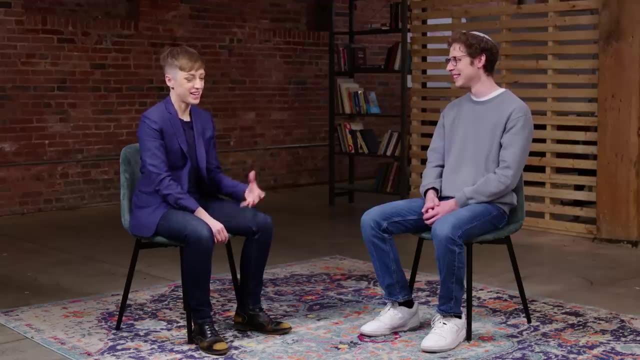 so clearly defined. What would you say a function is? I would say a function is a procedure that takes an input and does some operation and returns an output. That's the computer science brain thinking right there. So we want to think of a function as a procedure. 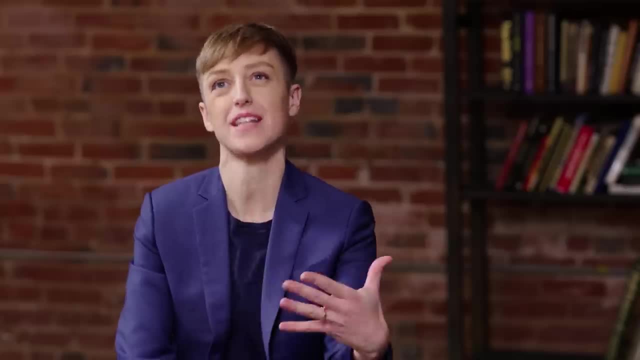 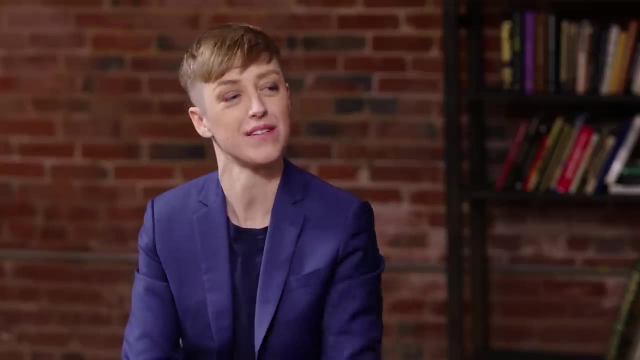 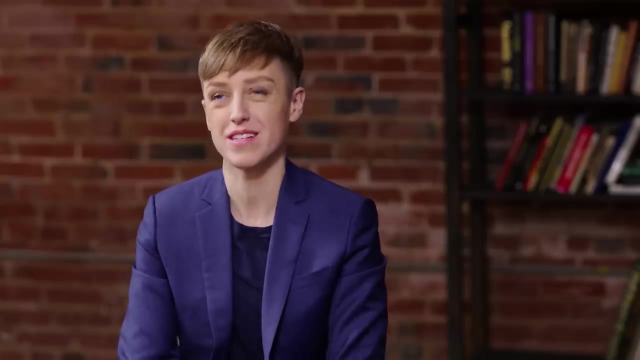 A procedure or a mapping between sets. So a function defines a one-to-one correspondence if it defines a perfect matching between the elements of its domain set and the elements of its output set. We call such functions bijections or isomorphisms. So the reason I'm so interested in this idea of a bijective function or a one-to-one correspondence. 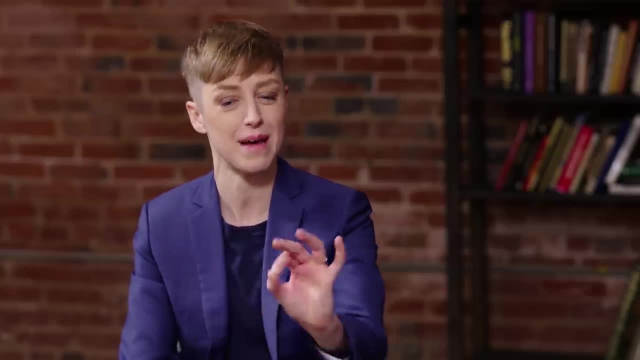 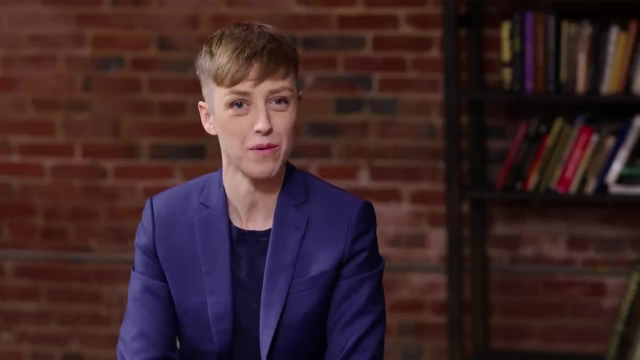 that guarantees that every element of one set gets matched with an element of the other set, no matter how many elements there are. These bijections, or these one-to-one correspondences, is they help mathematicians reason about infinity? How can you compare something that is endless? 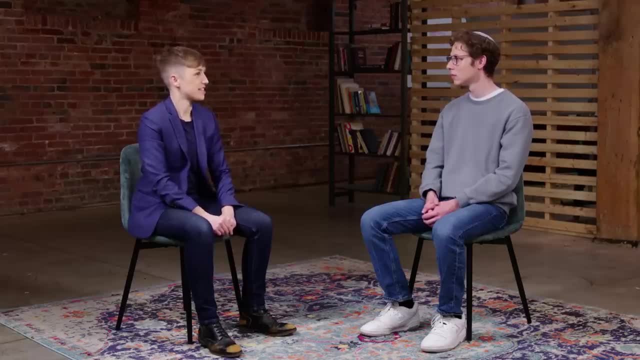 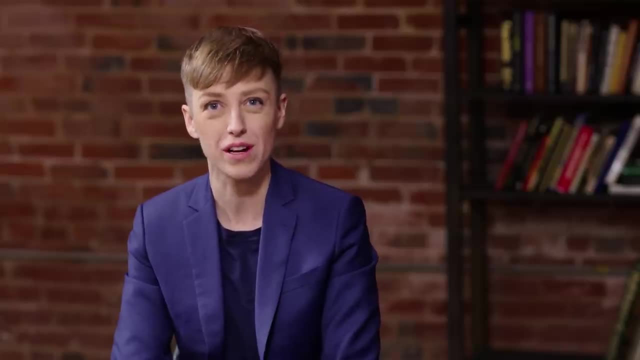 Today, we're going to think about infinity as a cardinality, which is a technical term for a number that could be a size of a set. We're going to use this idea of one-to-one correspondence to try and investigate the question of whether all infinite sets have the same size. 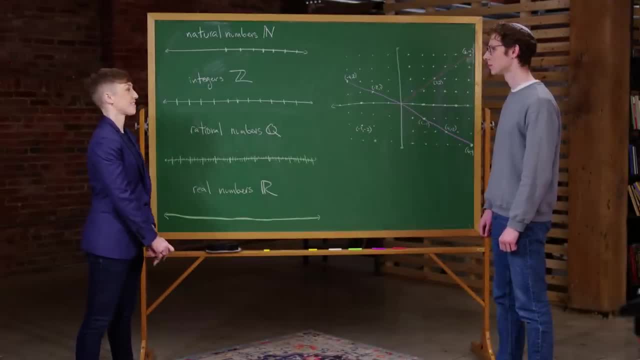 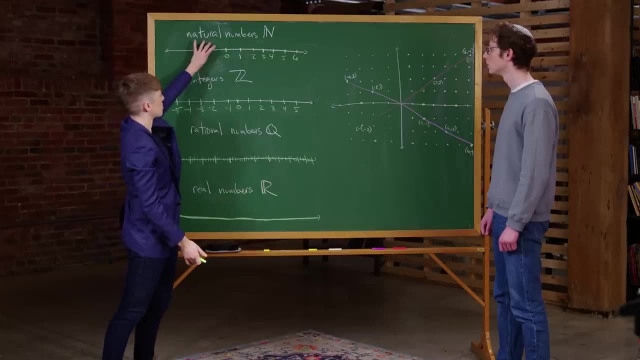 So what I've drawn here are some pictures of some of the infinite sets that appear in mathematics. So the natural numbers are the prototypical example of an infinite set. So the natural numbers are clearly a subset of the integers. Both of these are infinite sets. 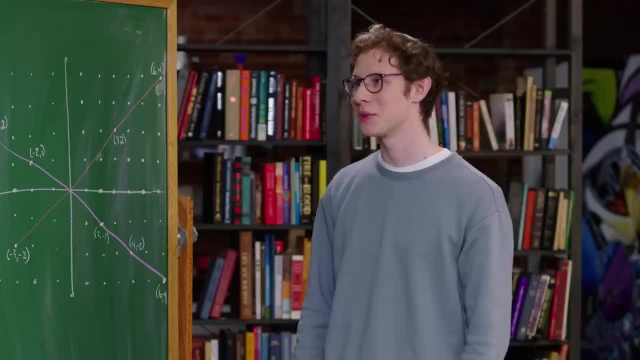 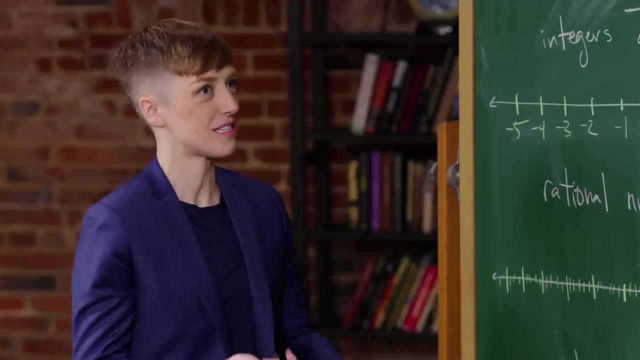 Are they the same size infinity or different size infinities? I guess the integers would. there'd be more integers than natural numbers. I'm going to now try and convince you that there are in fact the same size infinity, And this is using this idea of a one-to-one correspondence which was applied in this. 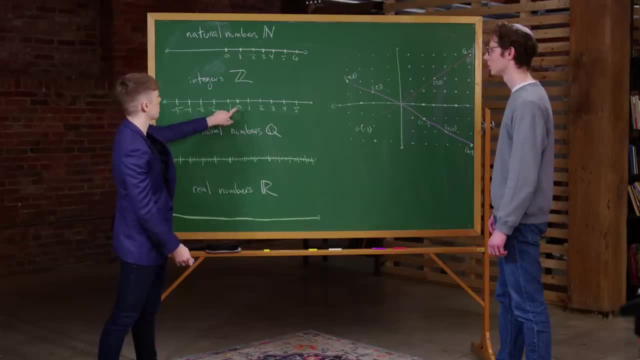 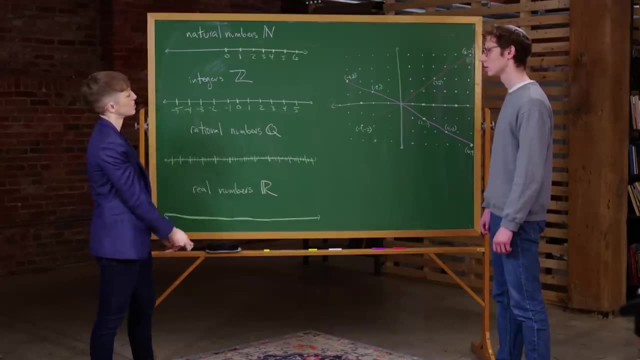 context by Georg Cantor. What he says is: if we can match up the elements of one set with the other set, then we're going to match up the elements of the integers with the elements of the natural numbers, so that there's nothing left over, so that there's a bijective function between them. 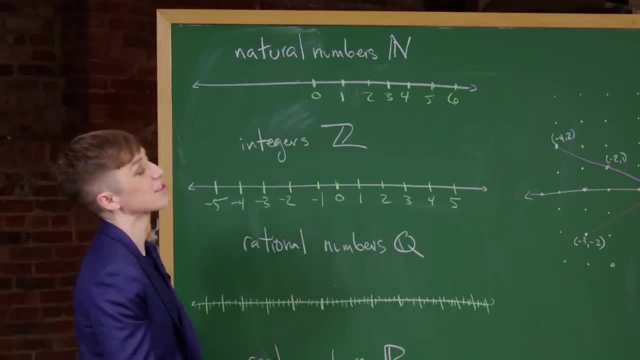 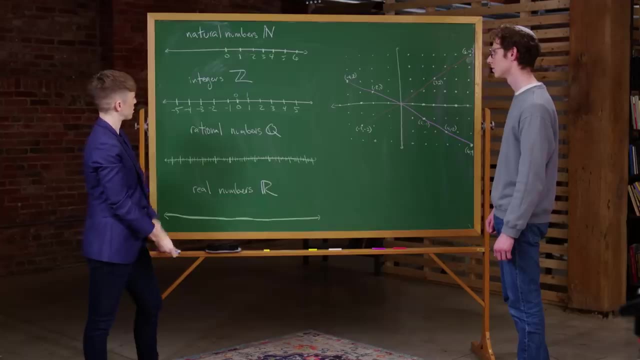 Then that's a proof that there's exactly as many natural numbers as there are integers. Start by matching zero with zero and one with one, But then we want to include the negatives in the list. So which natural number would we match with negative one? 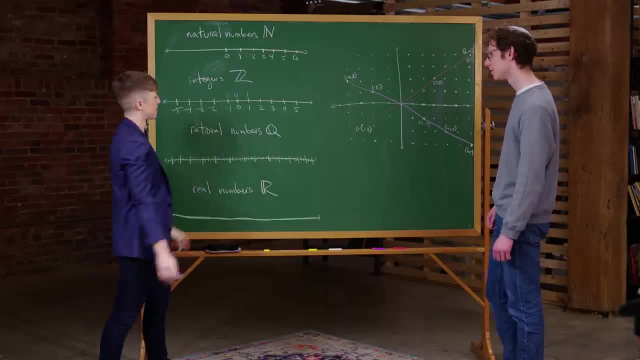 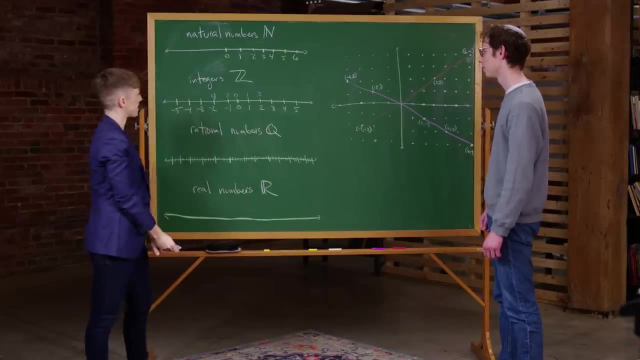 Maybe two, Maybe two. Why not? Because now we're starting to make progress on matching all the negatives. We can match the natural number three with the integer two, The natural number four with the integer minus two, And do you see a pattern? 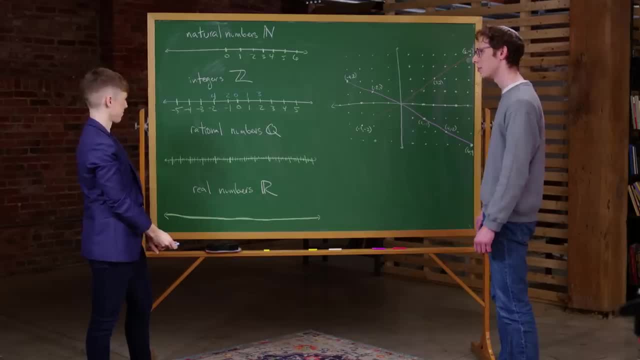 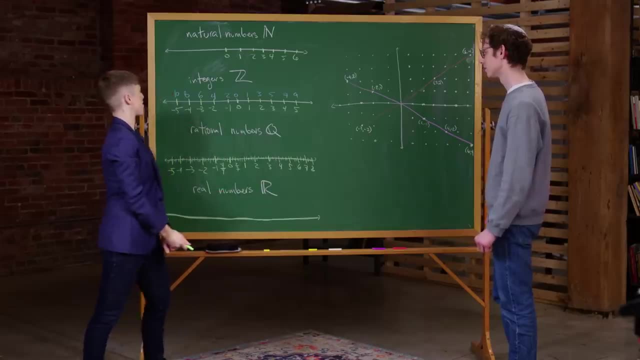 All of the positive integers would be odd numbers and all of the negative integers would be even numbers. Great. So now I have a much harder question. So we have the same challenge Again. evidently, there are way, way, way more rational numbers than there are integers. 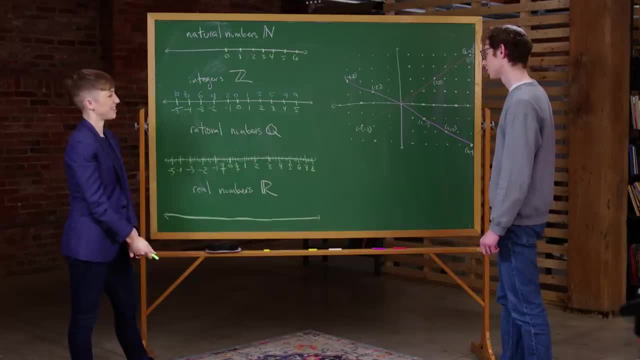 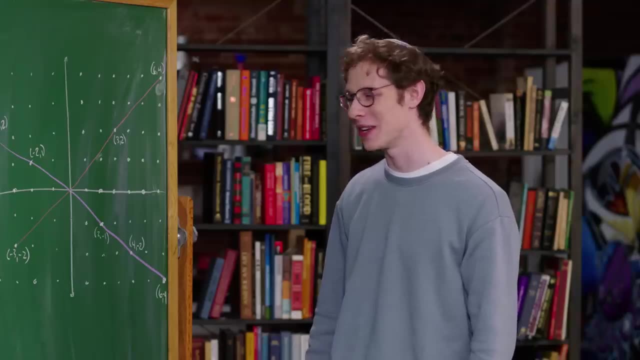 Does that mean this is a larger, infinite set than the integers? What do you think? By intuition I would say yes, But that was the same case with the integers. I would imagine there might be some bijective function for mapping natural numbers to. 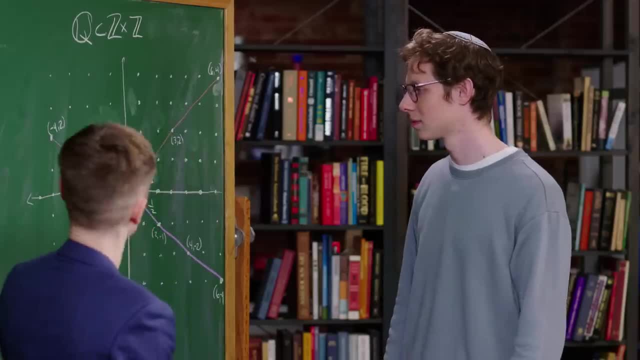 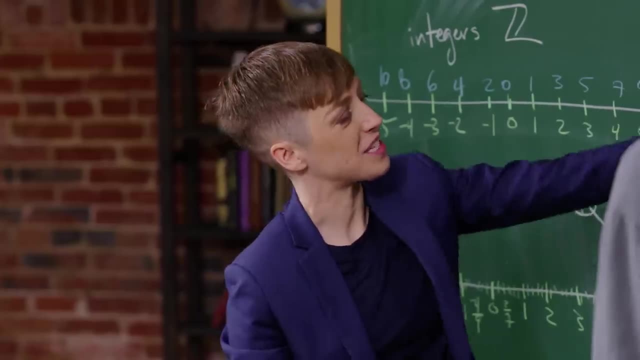 rational numbers. So I'm going to use this picture to count the rational numbers by actually counting the elements of this larger set, because it'll be clearer geometrically. What I've drawn in this picture is the integer lattice, So z cross z refers to the set of all of these dots. 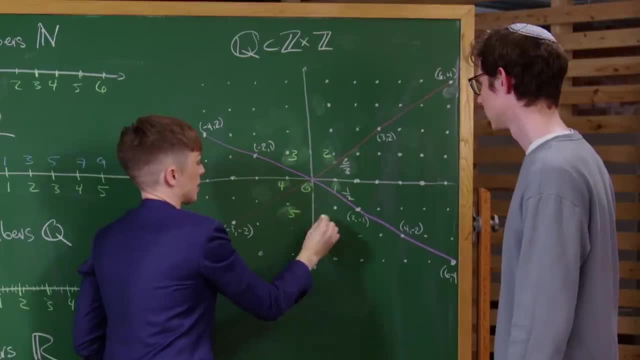 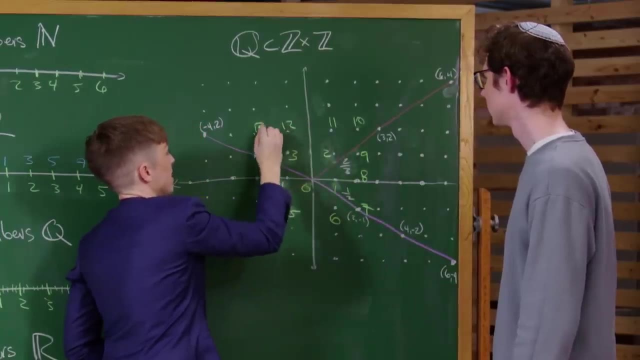 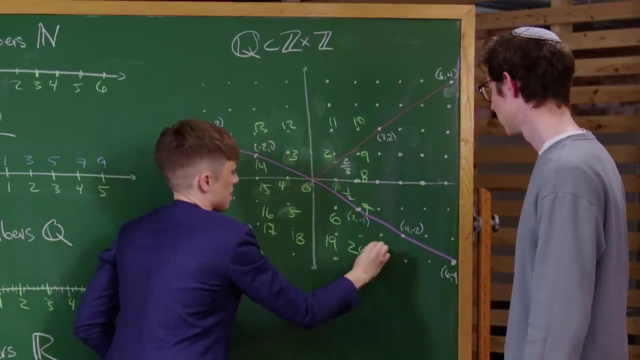 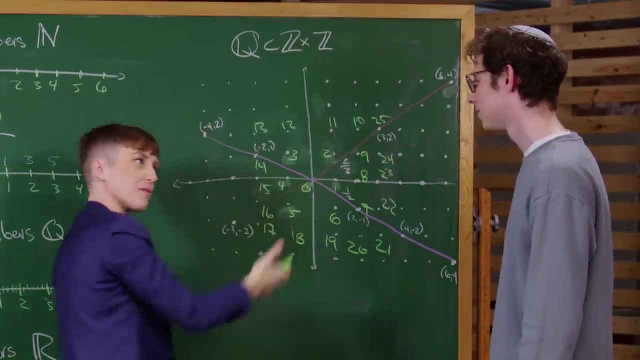 So I'll start by counting the number at the origin And you can see I'm just labeling the dots around the origin, moving in a counterclockwise fashion and getting progressively further away, And this process could continue. But maybe by now you see the pattern, though it'd be a little bit difficult to describe. 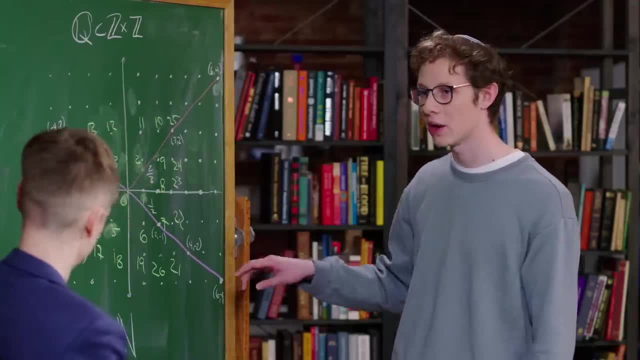 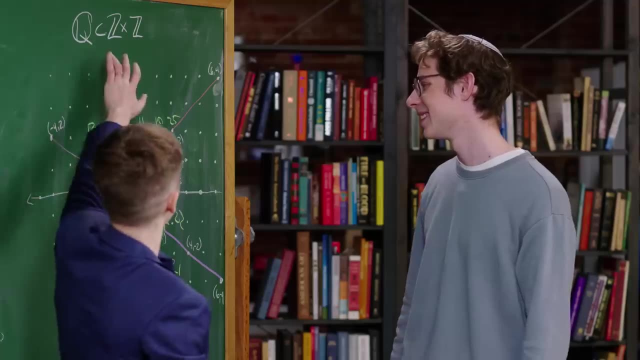 as a function. Oh, is it? for each rational number, there's a pair of integers that represent that rational number. Yeah, that's exactly right. And now, for each pair of integers, I'm going to represent it by a course, So I'm going to take the corresponding natural number. that's what's going on with this counting. 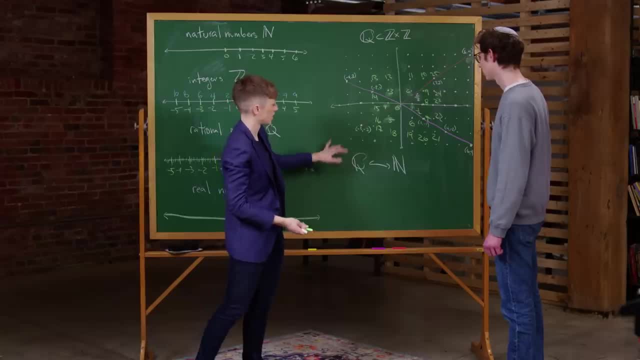 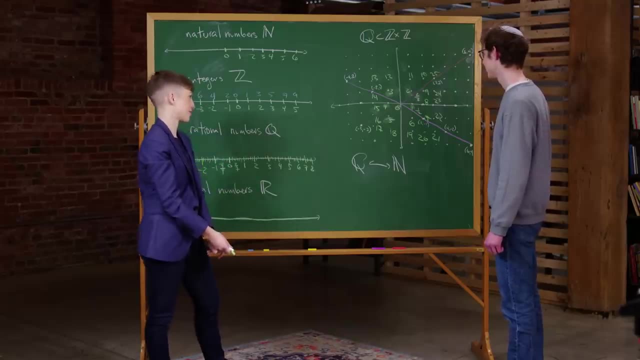 And when I compose those operations, what I've done is I've encoded rational numbers as natural numbers in a way that reveals that they can be no larger. There are no more rational numbers than natural numbers. So this slope is represented by 3, 2, and 3, 2 is in here as 25, don't you? 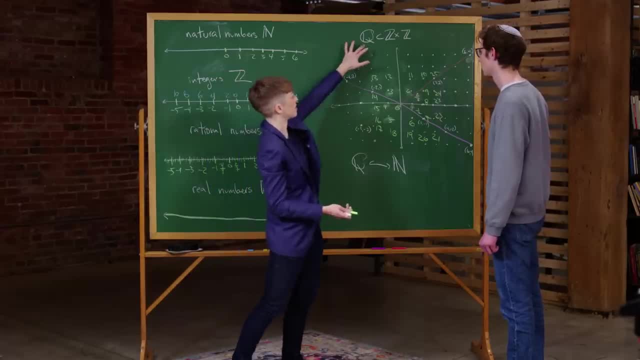 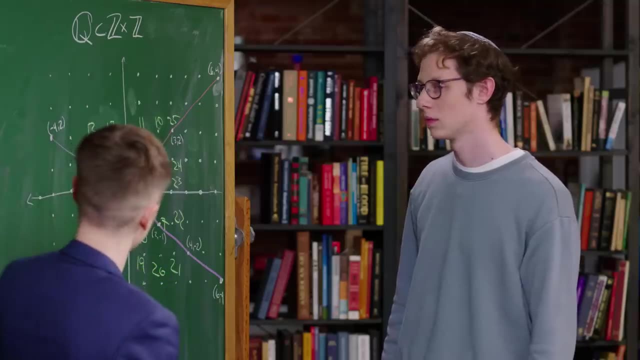 Exactly, That's exactly right. So we were hoping to compare the size of infinity of the rational numbers with the size of infinity of the natural numbers. So what we've done is introduced an intermingling, We've introduced an intermediate set, these pair of integer points. 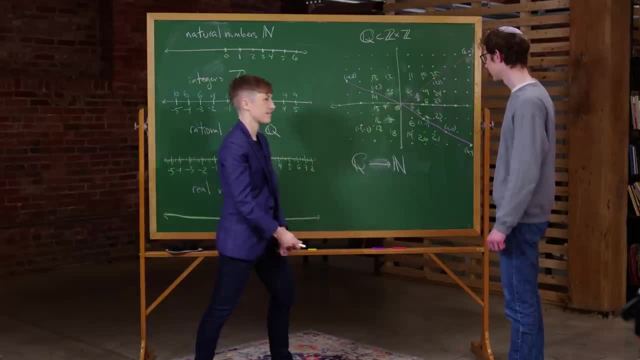 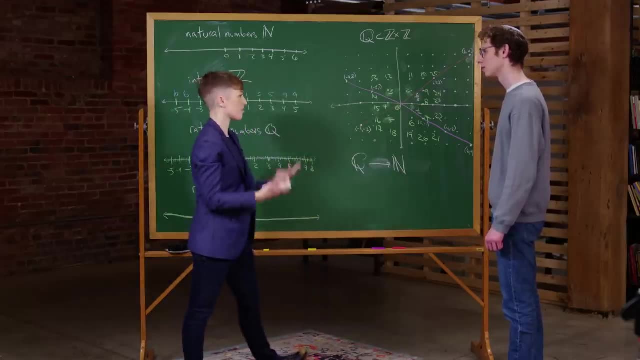 And this proves that this size of infinity is smaller than this size of infinity, Since we also have an injective function. the other way, this size of infinity is smaller than this size of infinity, so therefore they must be the same size. That's wild. 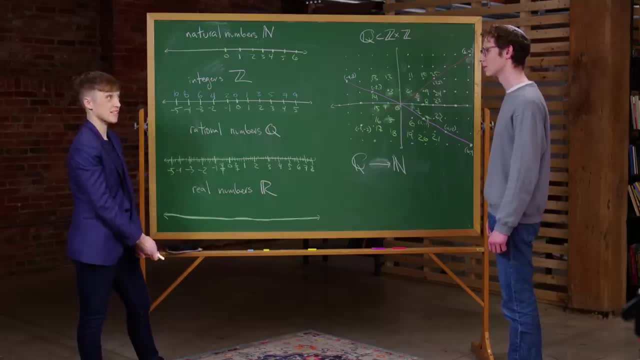 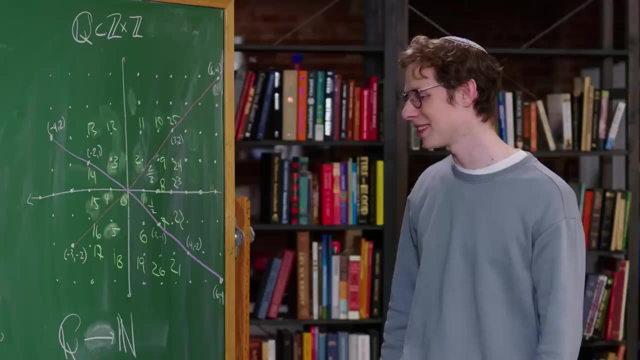 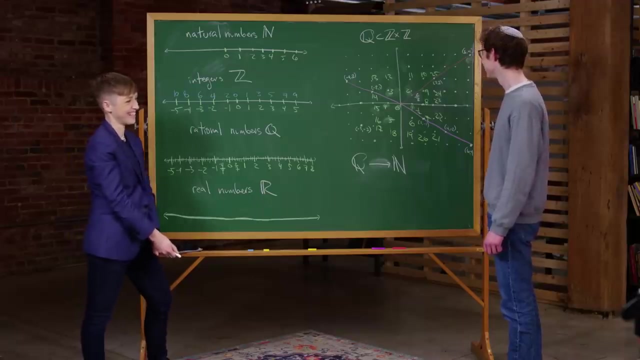 Now there's one final collection of numbers that we haven't yet discussed, which are the real numbers, all of the points on the number line. Do you think that's the same size? infinity, I guess? I mean it seems like it must be much larger, but I don't know. I haven't been on a roll. 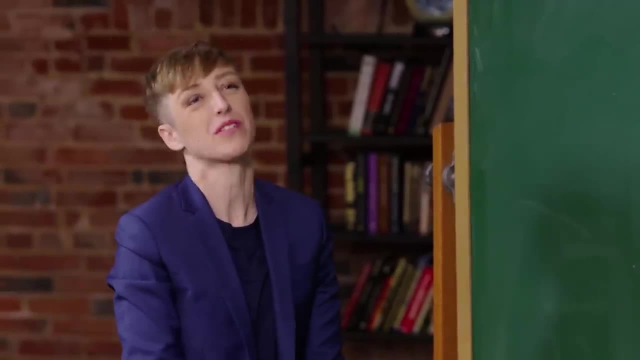 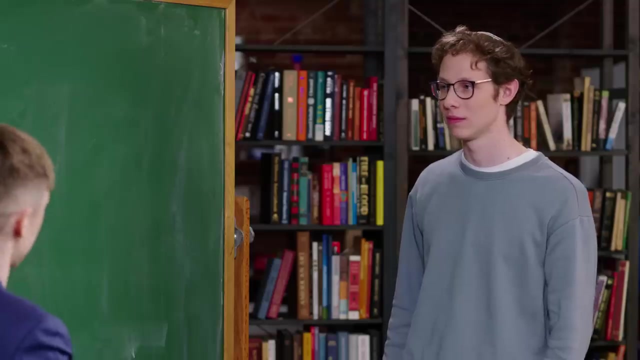 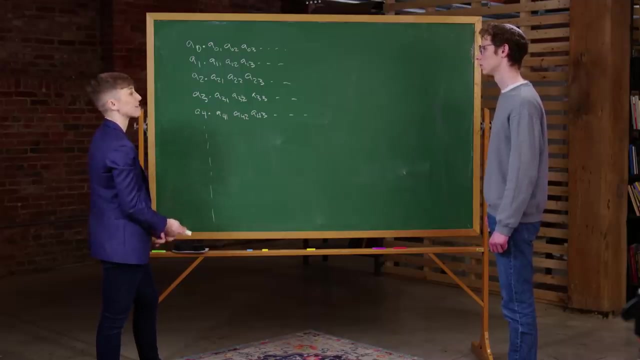 Georg Cantor proved that it is impossible to count all real numbers like we've just counted the rational numbers or just counted the integers. This is called the cardinality of the continuum: is uncountable. What I'm going to do now is form a new real number that I guarantee is not on this list. 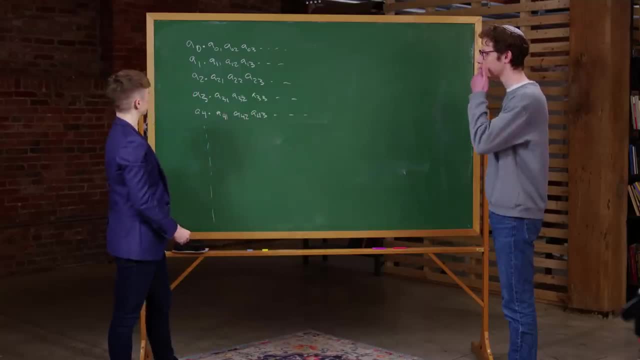 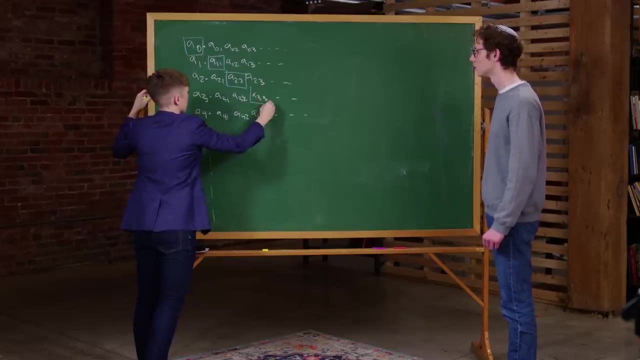 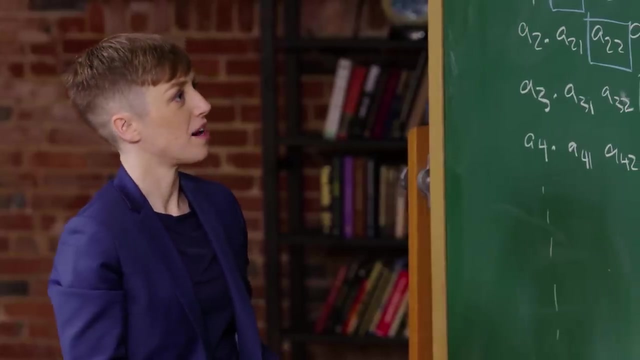 So here's how we do this. What I'm going to do is I'm going to look at the diagonal, So I'll highlight them. This continues forever, And now I'm going to form a new real number by changing all of these digits. 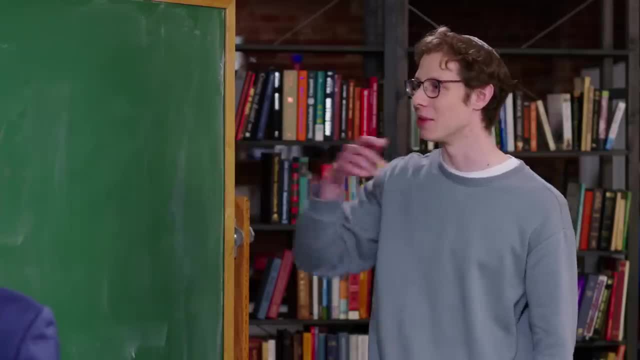 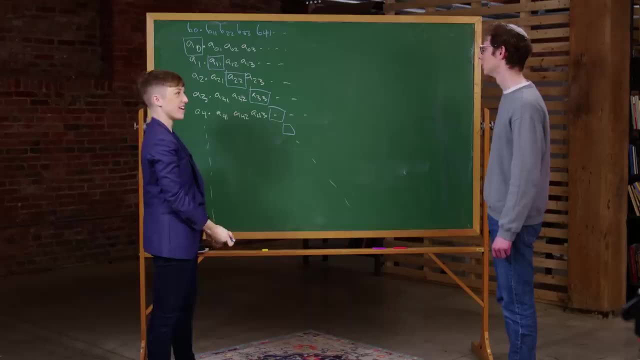 If you just like, added one to them, then that would be something that doesn't exist in any of the other ones. Yes, You see the idea right away. So I'm going to form a new real number whose first digit is different from this one, and 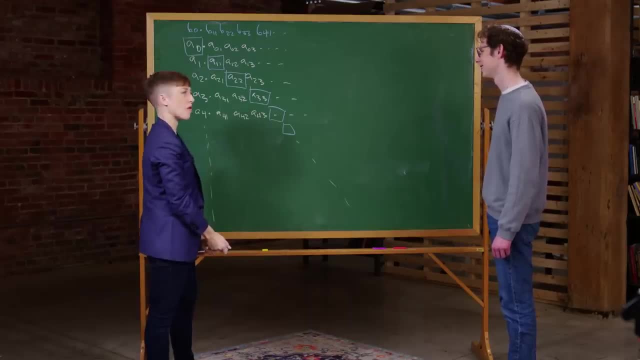 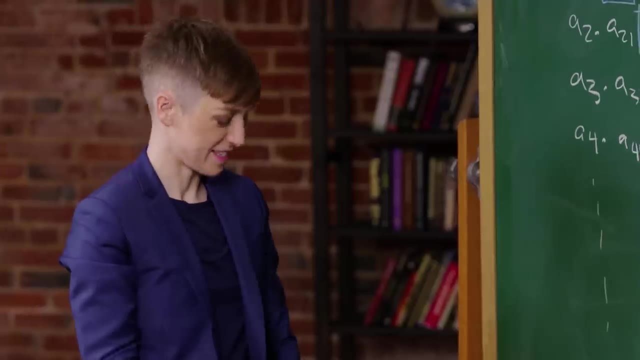 you've already convinced me, You've convinced yourself that this number is not on this list anywhere. Why is that? Because at every point there's at least one change from a number in there. Great, That's exactly right. So what we've proven is that this number is missing and therefore it is impossible to 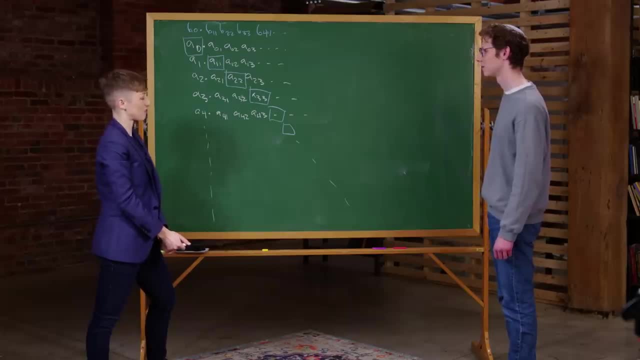 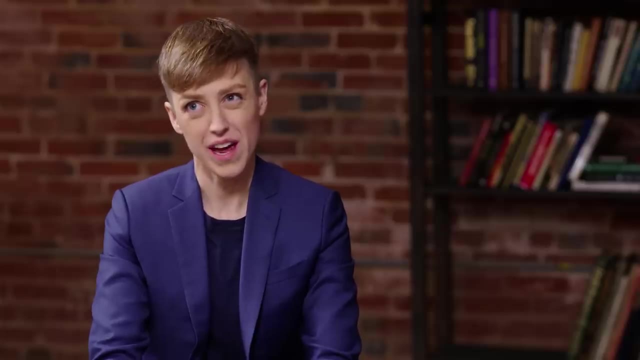 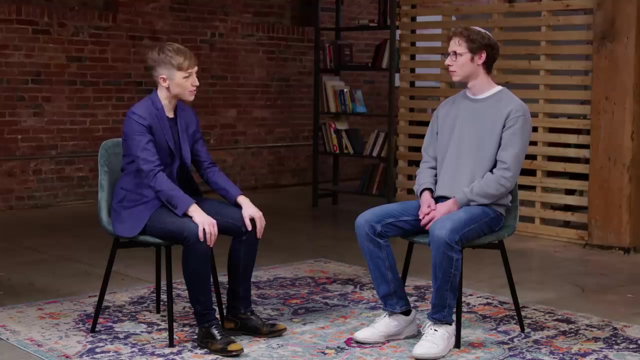 define a bijection between the natural numbers and the real numbers. So we've started to explore some of the counterintuitive properties of infinity. On the one hand, there are infinite sets that feel very different, The natural numbers, the integers, the rational numbers that nevertheless have the same. 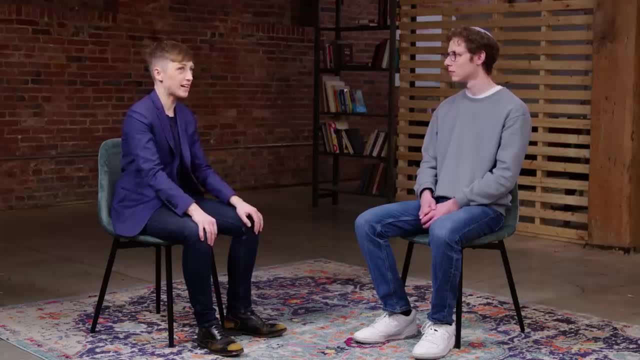 size or the same infinite cardinality, while there are other infinities that are larger, So there's more than one size of infinity. Not all infinities are created equal. I was wondering what the kind of practical implications are, what you can do with this. 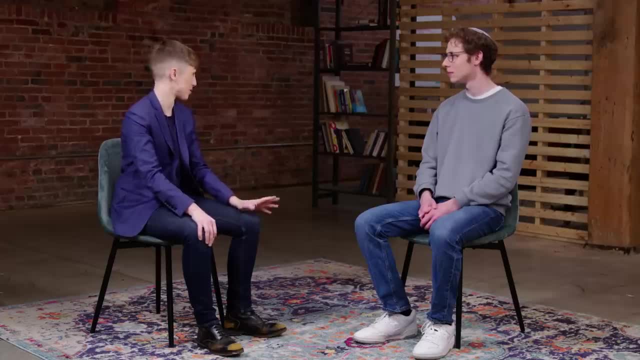 sort of knowledge. I'm really glad you asked me that There's a practical implication for computer science. Alan Turing. he came up with a mathematical model of a computer, something called a Turing machine, And he was wondering: is it possible to compute every real number, an arbitrary real number? 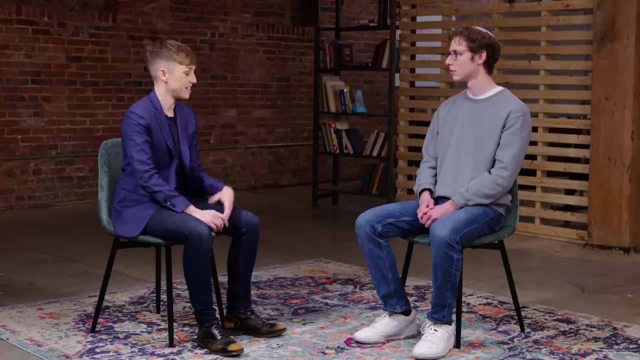 to within arbitrary precision in finite time. He defined a real number to be computable, if you could calculate its value, maybe not exactly, but as accurately as you'd like, in a finite amount of time. And because there are uncountably infinitely many real numbers, but only countably infinitely. 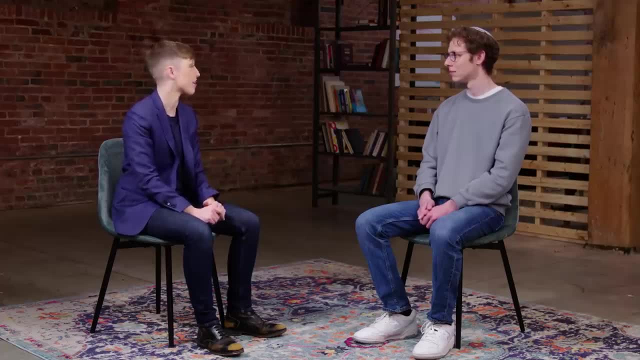 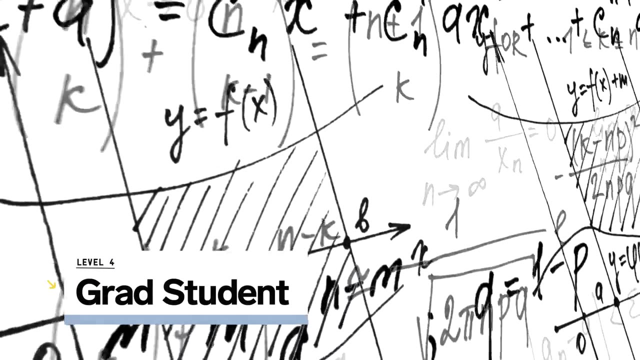 many Turing machines. what that means is that the vast majority of real numbers are uncomputable, So we'll never be able to access them with a computer program. You're a PhD student, Is that right? Yes, I'm a second year PhD student at the University of Maryland. 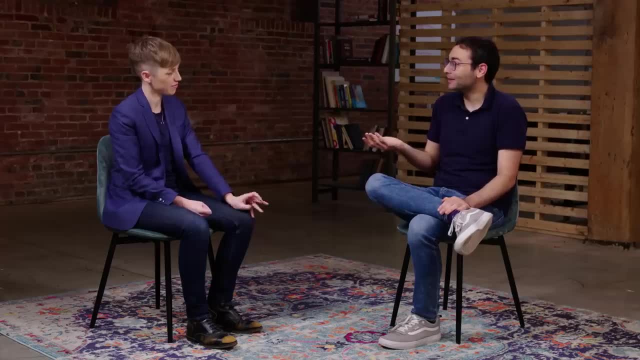 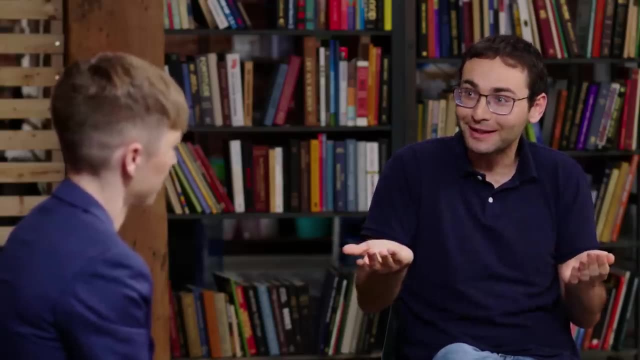 Does infinity come up in your mathematics that you're studying? One place infinity comes up is in algebraic geometry. Normally we think, okay, well, if you have two lines like this, you'd keep drawing them while they intersect right here. But in projective space, two parallel lines will also intersect at the point at infinity. 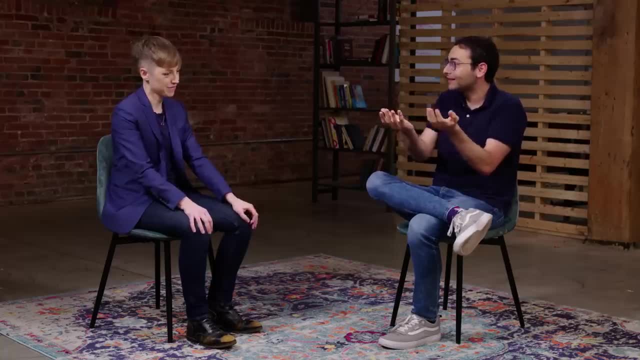 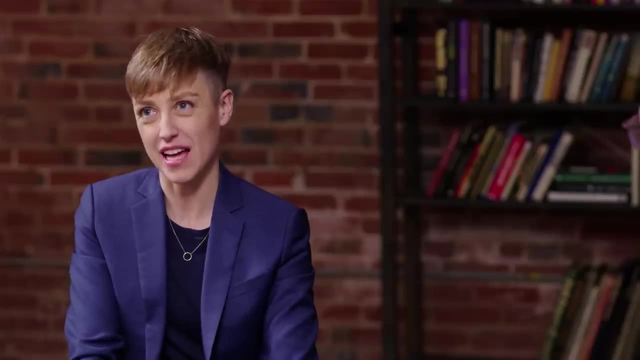 Infinity is like this: perfect concept for what we can add to a space that allows lines to have this more uniform property. What's your research in? So one of my main research areas is something called category theory. It's been described as the mathematics of mathematics. 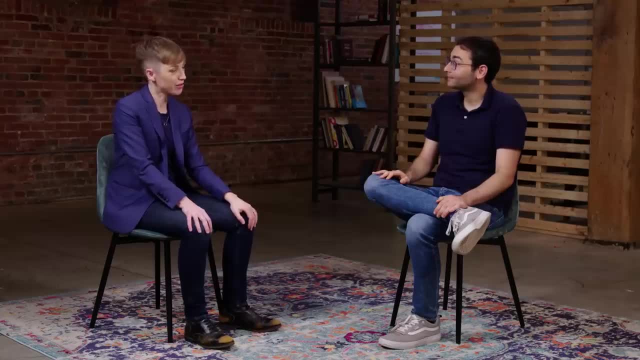 It's a language that can be used to prove very general theorems, And an interesting aspect of being a researcher in category theory that doesn't come up as much in other areas is that we have to really pay attention to the axioms of set theory. 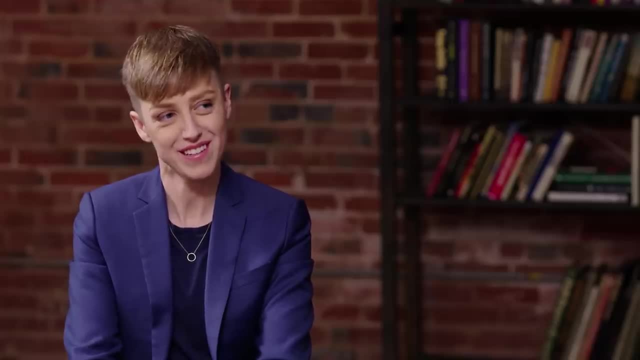 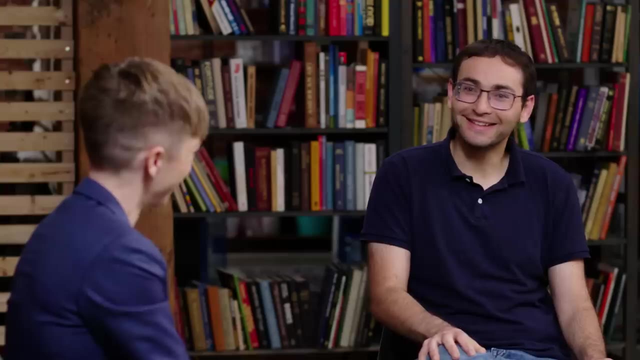 in our work, When you're proving theorems, have you ever used the axiom of choice? Yeah, It's basically this idea that you can put a choice function on any set And a choice function does what exactly? Yeah, that's a good question. 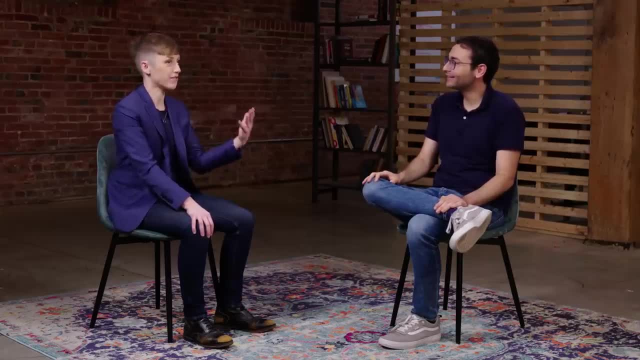 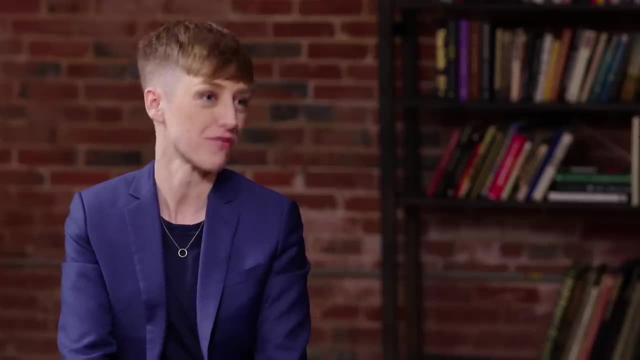 So the way I think about it is, if you have an infinite or an arbitrary family of sets and you know for sure that none of these sets are empty, then a choice function would allow you to select an element from each set, sort of all, at once. 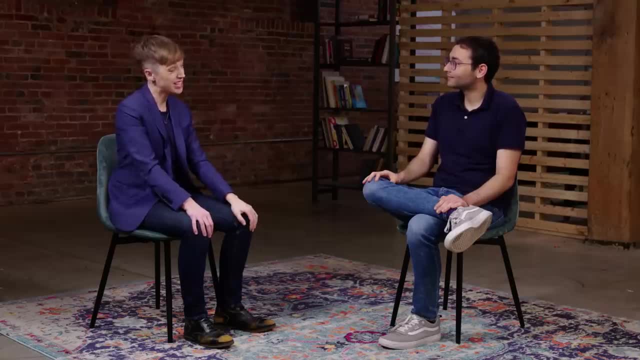 When you've used the axiom of choice in proofs. do you know which incarnation of this you've used? Yeah, I've used it like that. I've also used it in Zorn's lemma. What about the well-ordering principle? So there are three well-known, famous equivalent forms of the axiom of choice. The well-ordering principle is the assumption, the axiom that any set can be well-ordered, But there are lots of subsets of real numbers that do not have a minimal element, so that ordering is not a well-ordering. So here's the key question. 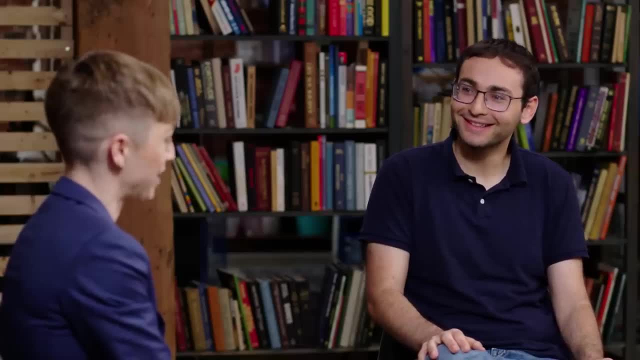 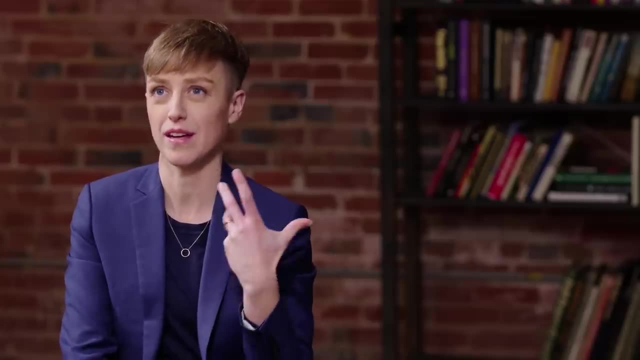 Do you believe the axiom of choice? I do believe the axiom of choice. You do believe the axiom of choice, though it leads us to some strange conclusions. So if the axiom of choice is true, then it's necessarily the case that there exists a 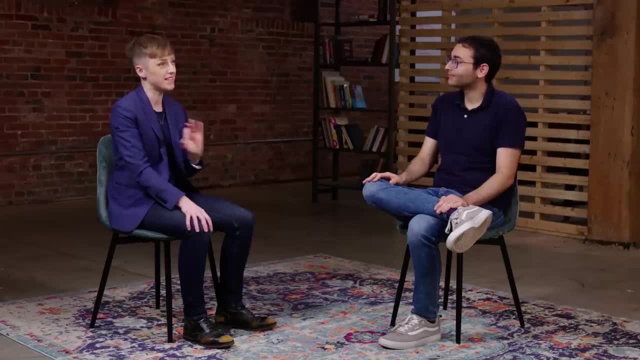 well-ordering of the reals, And what that means is that we can perform induction over real numbers like we perform induction over the natural numbers. This is transfinite induction. It would work for any ordinal, So there must be some uncountably infinite ordinal that represents the order type of 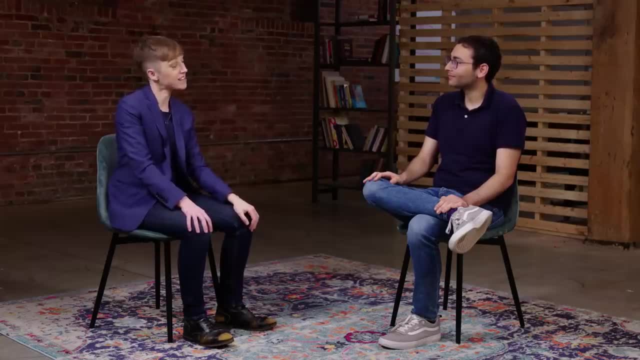 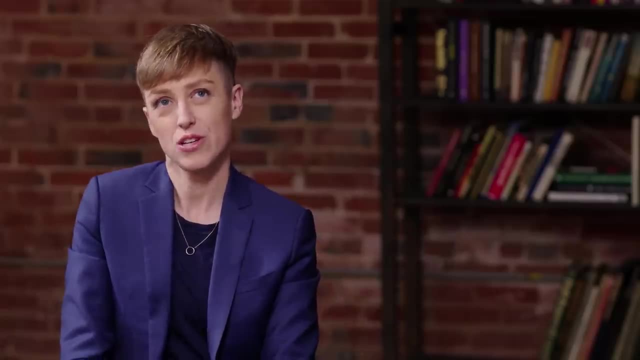 the real numbers, And this allows us to prove some crazy things. Imagine three-dimensional Euclidean space, So the space that we live in, Extending infinitely in all directions. So it is possible to completely cover three-dimensional Euclidean space by disjoint circles. 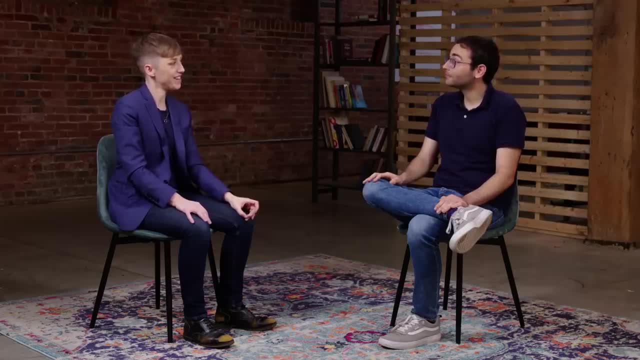 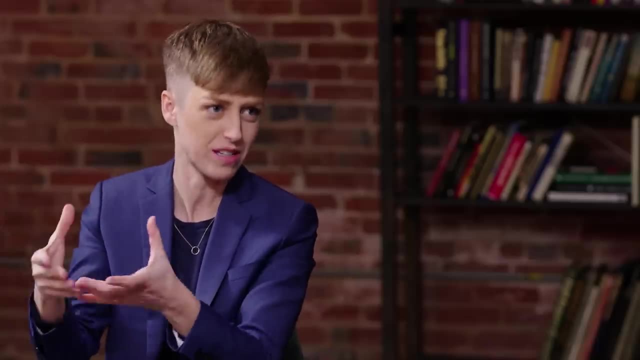 So infinitesimal circles disjoint circles of radius one. So what that means is you can put a circle somewhere in space and then put a second circle somewhere in space that can't intersect with the first one, because these are solid circles- and then another circle and somehow cover every single point in space with no gaps in. 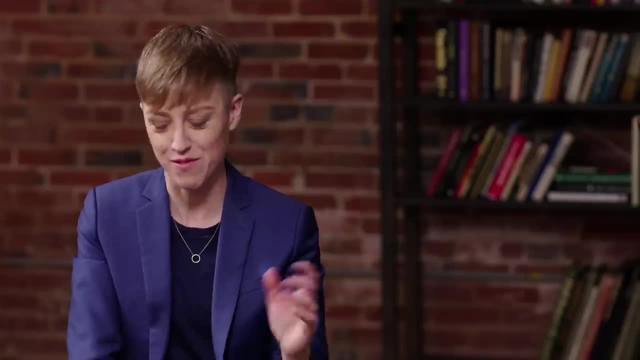 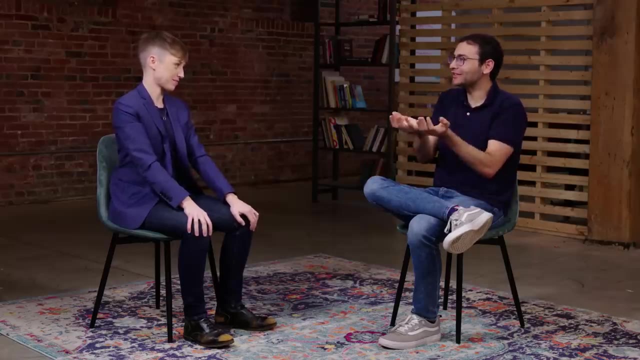 between. That's crazy. Yeah, That's a crazy thing. Do you have a favorite consequence of the axiom of choice? I mean, the Bonn-Oktarski paradox is a big one. So basically it says that you can using just rigid motions. I think you can take one ball. 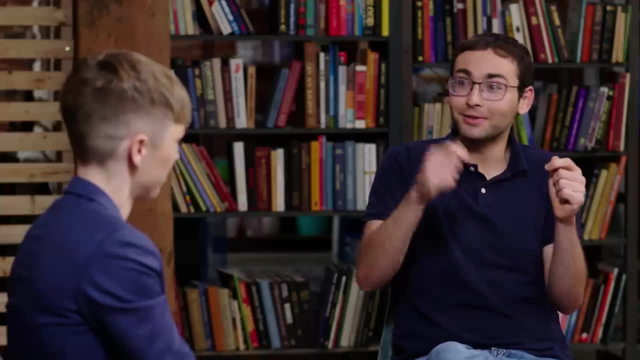 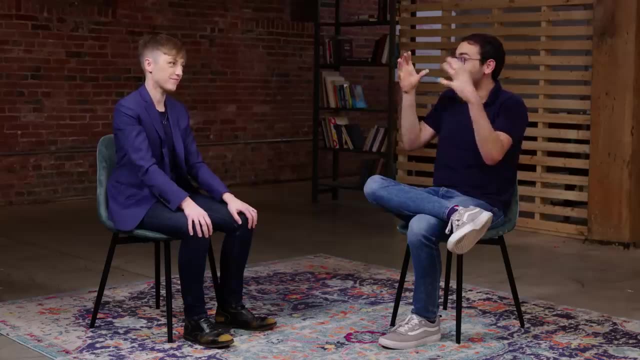 cut it up, One solid ball with a finite volume. Yeah, Cut it up and then rearrange the pieces so that in the end you get two balls which are the exact same size, the exact same volume. So you've actually taken one thing and using just pretty normal operations to it, you can. 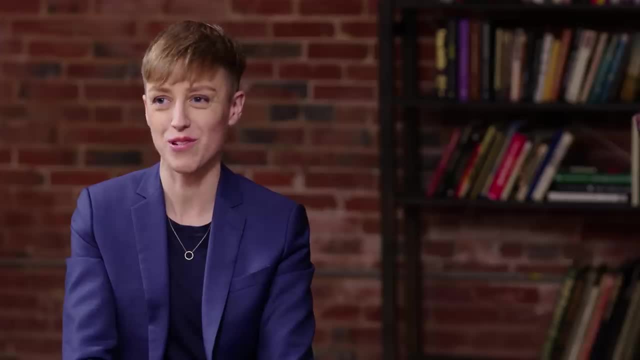 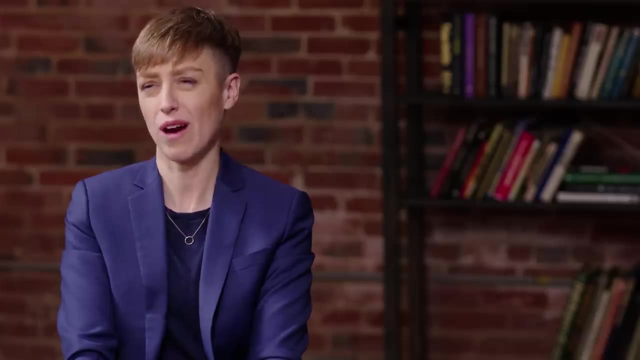 double it, which seems pretty implausible in real life, Right? That seems crazy to me. That's irrefutable consequence of this axiom that you tell me you believe is true. Yeah, So how many infinities are there? Well, definitely uncountably many infinities. 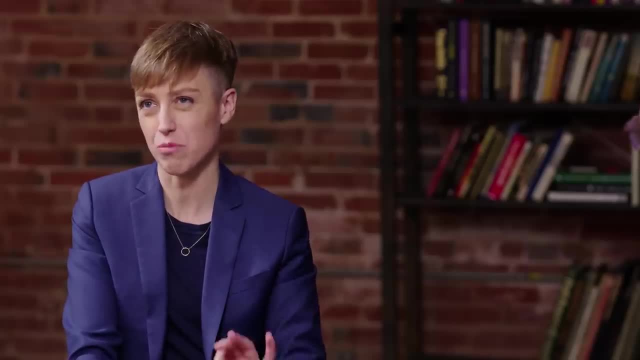 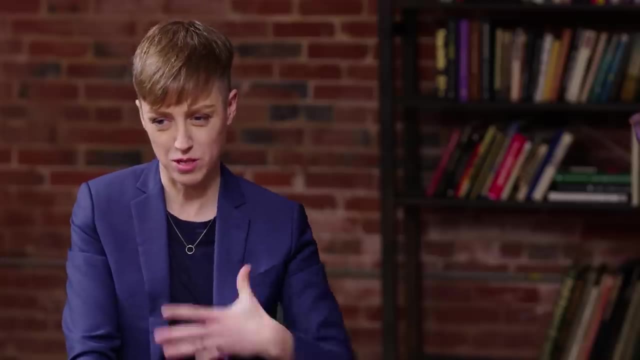 Right. So there's no, there's certainly no stop to this procedure. but could you give a precise cardinality to that? Probably not, because if I could, there would be a set of all sets right. So Cantor's diagonal argument can be abstracted and then generalized to prove that for an 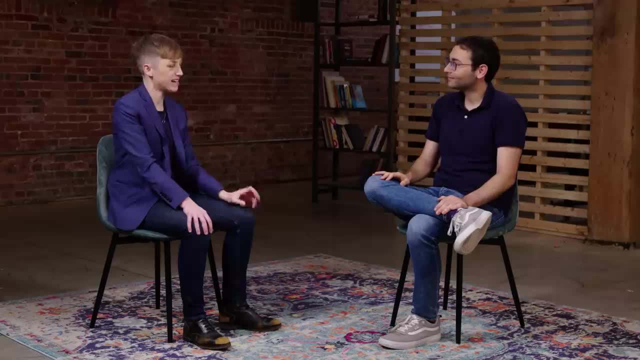 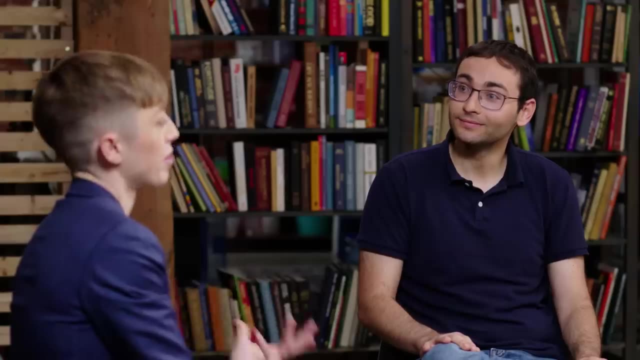 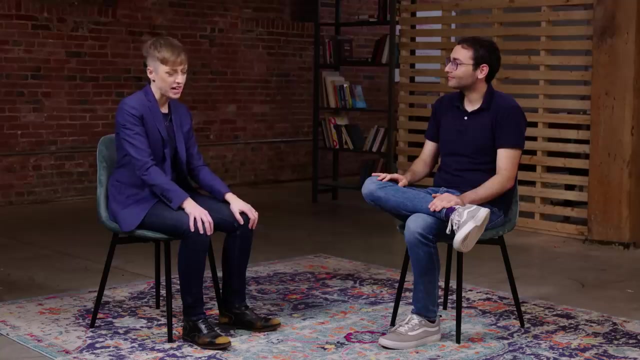 arbitrary set A. its power set has a strictly larger cardinality, And since that's true for any set, we can just iterate this process When set theory was being discovered or invented or created in the late 19th century. one of the natural question to ask is: can there be a universe of all sets? 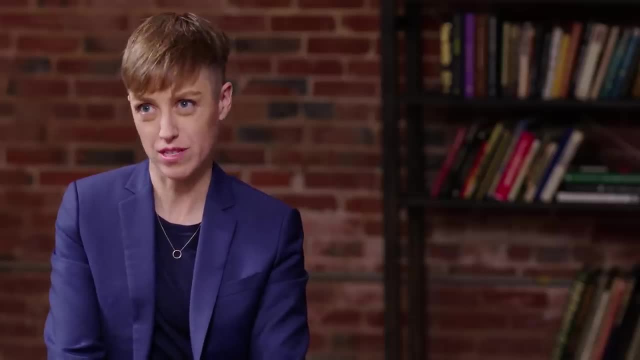 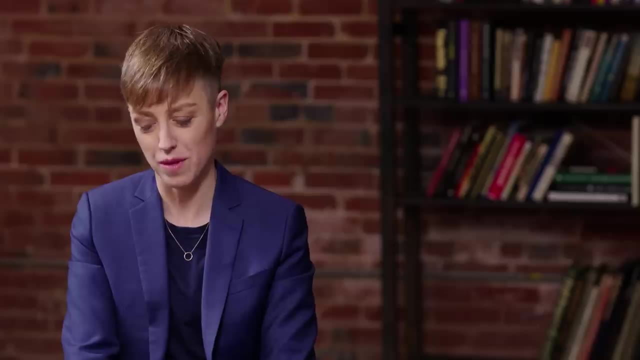 This comes up in my research in category theory, because even though there is no set of all sets, we would really like for there to be a category of sets. So what category theorists need to do to make their work rigorous is to add additional axioms. 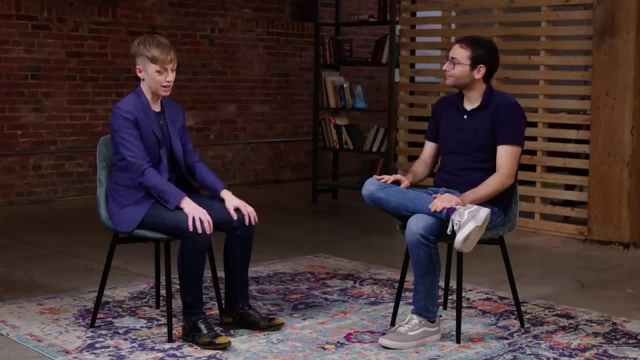 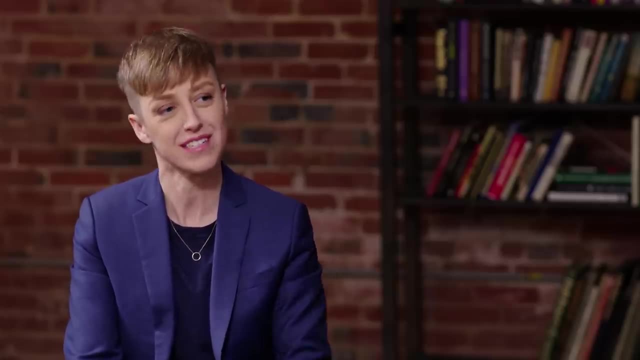 to set theory. One of my favorites was introduced by an algebraic geometer, Alexander Grothendieck. This is something that we sometimes call a Grothendieck universe, or also an inaccessible cardinal. It's an infinite number that is so big that it cannot be accessed by any of the other. constructions within set theory. It's so big that we'll never get to it, And this allows us to contemplate the collection of all sets whose cardinality is bounded by this size that we'll never reach. So you're just making a cutoff point. You're saying we're never going to get sets bigger than this anyway, So we might as well make our category only include things smaller than that. That's right. So a rigorous way to work with a category of sets is to demand that it's a category. 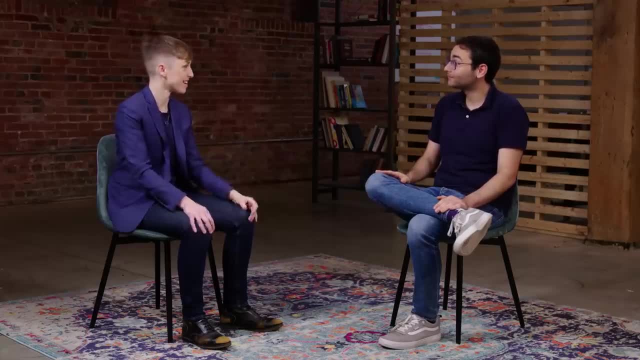 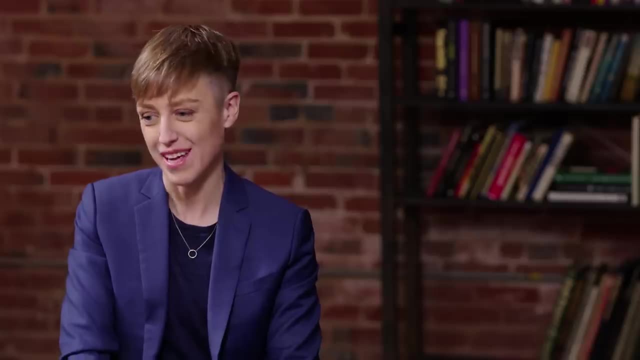 of sets whose size is bounded by this cardinality, alpha say. That is then an example of a category that fits into another still larger growth in the universe: beta. So implicitly in a lot of my research, I have to add an additional assumption: that 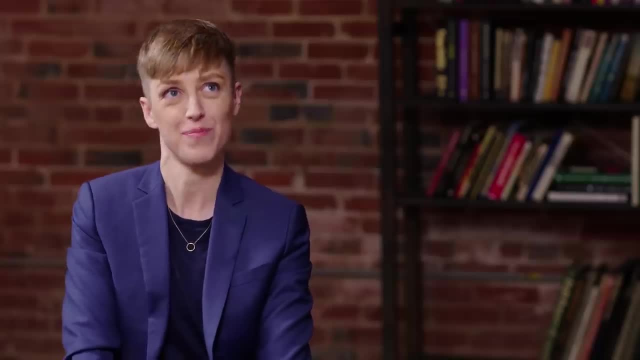 there exist maybe accountably many inaccessible sets, And that's what I'm trying to do. I'm trying to make sure that I'm not making a cutoff point. I'm trying to make sure that I'm not making an inaccessible cardinals. 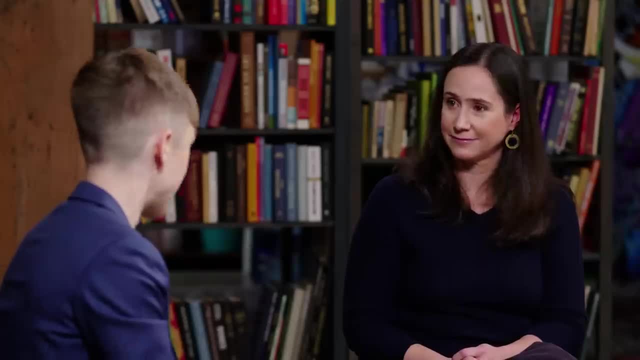 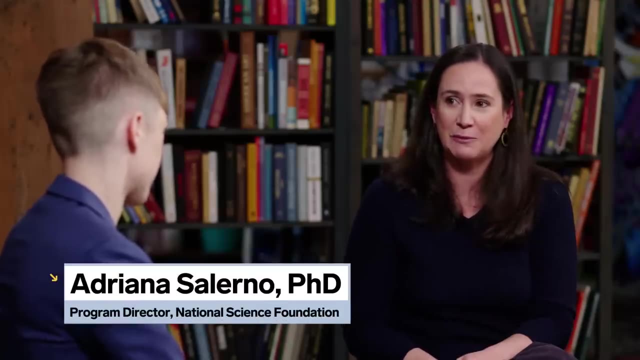 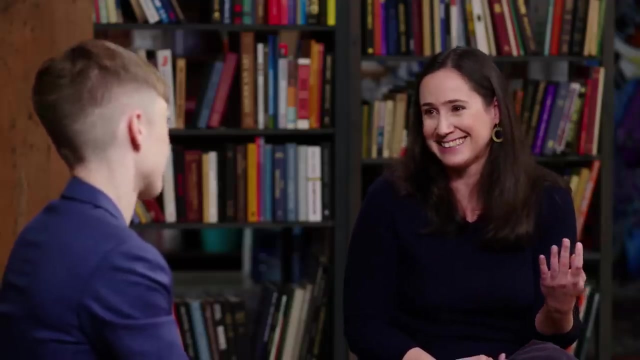 Examples of infinite sets abound in mathematics. We see them every day. So do those infinities exist? I think you'll get a different answer from every person, every mathematician you meet. It is a construct, So it exists, in the same way that things like that, like that poetry, exists when you talk. 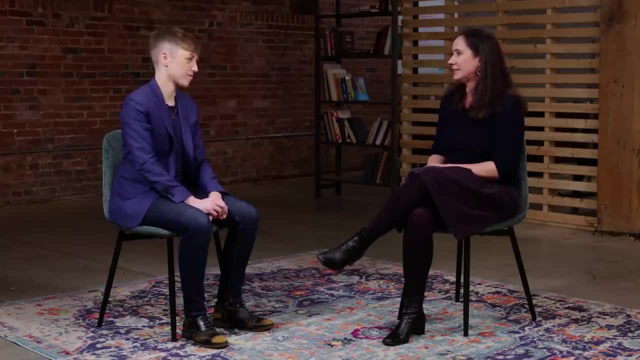 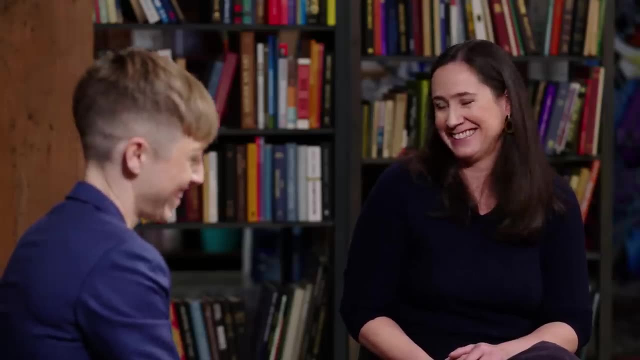 about even cardinality, And it's just like: well, here's an infinite hotel. I had one student who was like no, no, it does not exist. When I describe like well, imagine you do this infinitely many times. 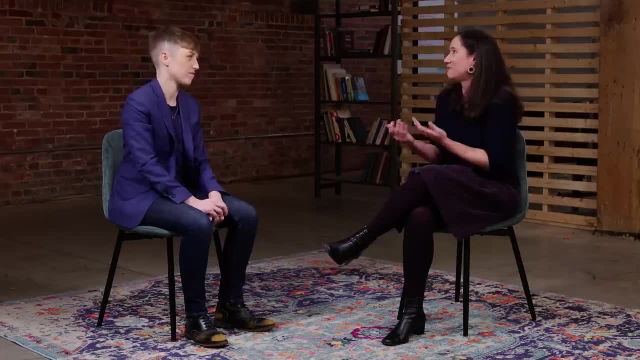 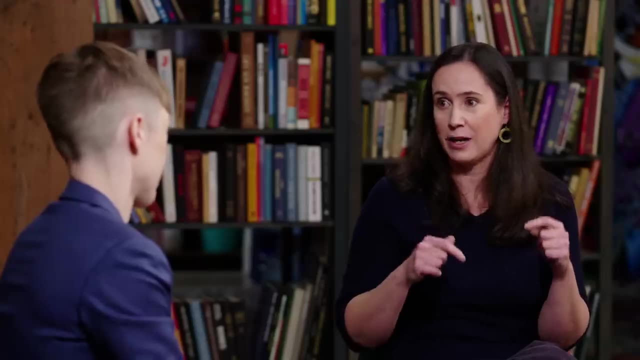 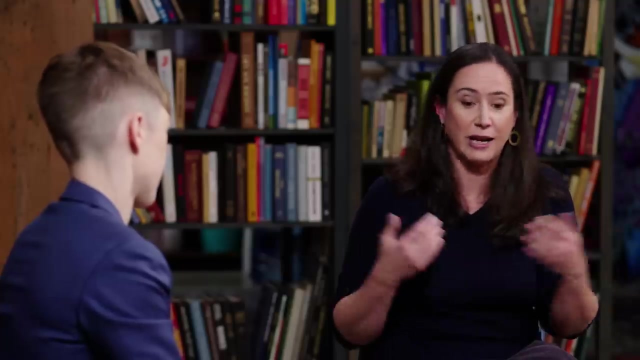 They're done with me because they're like I can't. No one can do this infinitely many times right? These interesting paradoxes that come from like the ape typing in a typewriter and eventually getting to Hamlet is an example of like well, if you give something forever and any random. 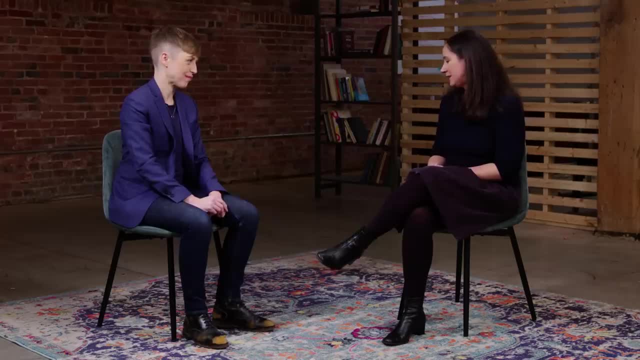 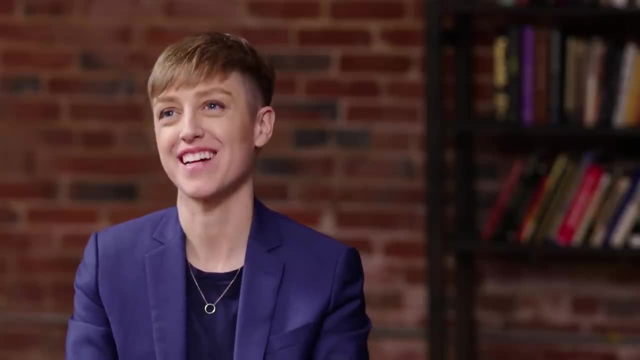 event is going to happen. It can be generative for sure. It's definitely a really interesting, really interesting thing to try to talk to students about. I mean, I'll grant you that Hilbert's Hotel does not exist. For me, infinite objects absolutely exist. 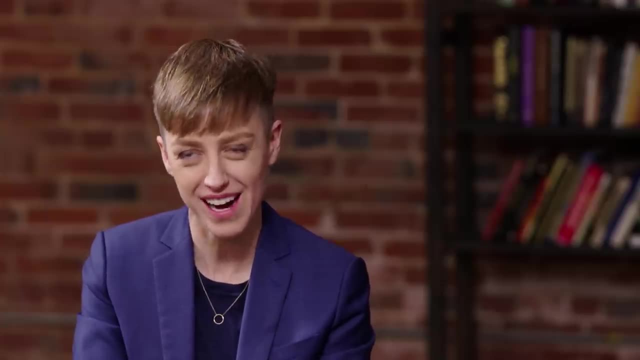 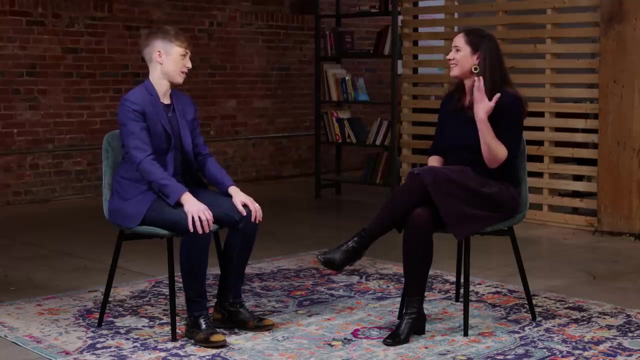 And I can't read the thoughts in your head, but I have a high degree of confidence that we have a lot of the same ideas about infinity. It's this idea that are things that you can think of. do they exist? You're getting into philosophy of math now, which is exciting. 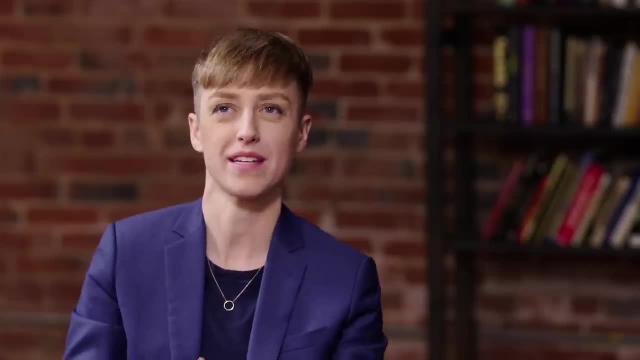 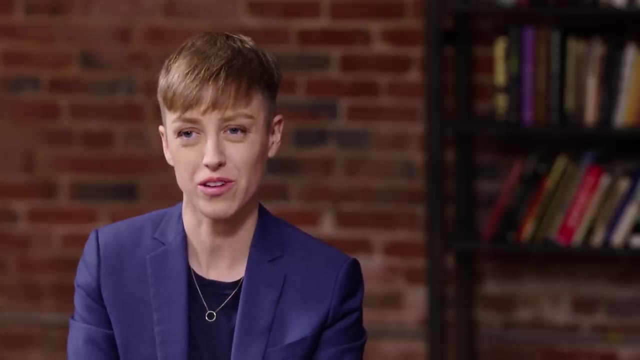 I mean, I think that's great, I mean I think that's. another common misconception about mathematics is that it's so far removed from the humanities, for instance. It's hard to ignore some of these philosophical questions, particularly when we're talking. 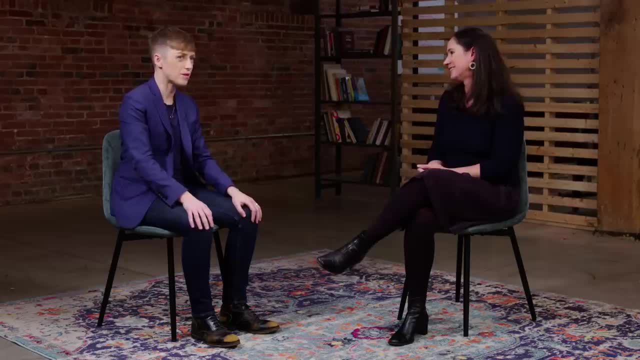 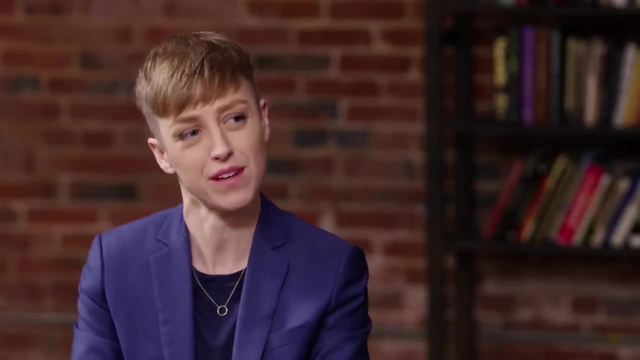 about certain things like infinity, And I think one of the most difficult things to really be precise about and to explain to students is the continuum hypothesis. What do you say to students about the continuum hypothesis? The most fun thing to teach when you teach about infinity, when students realize that. 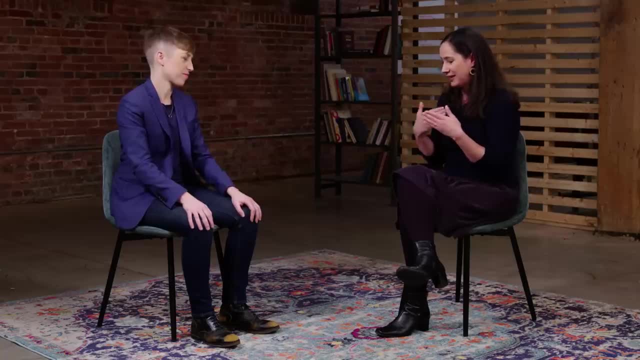 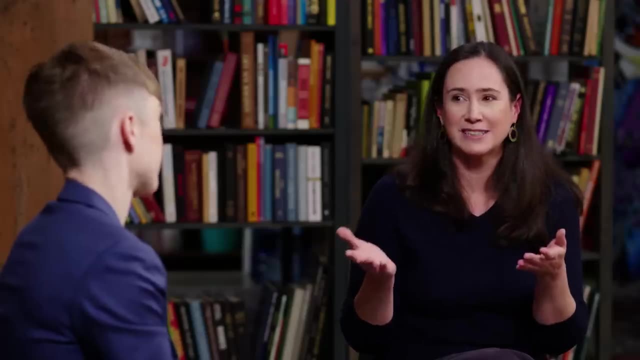 you are talking about different sizes of infinity, Mm-hmm, And a natural thing is for them to think about, like what is the next size of infinity that I can think about? And sort of the continuum hypothesis is sort of one of these really hard things to grasp. 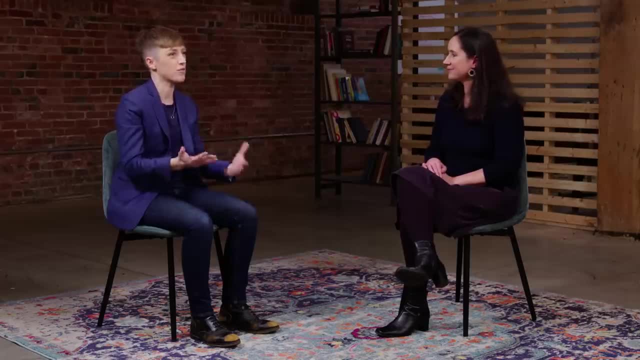 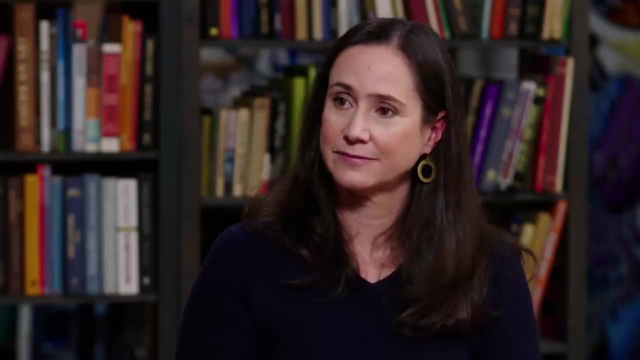 So what's so fascinating about the continuum hypothesis? if you take a subset of the real line that's infinite, does it necessarily have either the cardinality of the naturals or the cardinality of continuum, or is there some sort of third possibility? 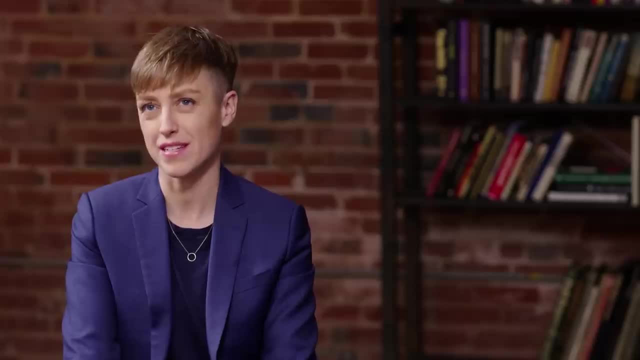 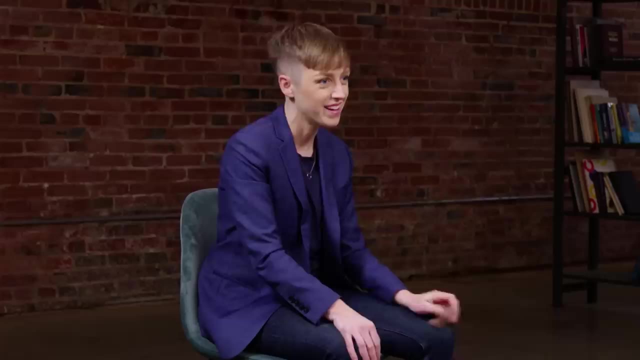 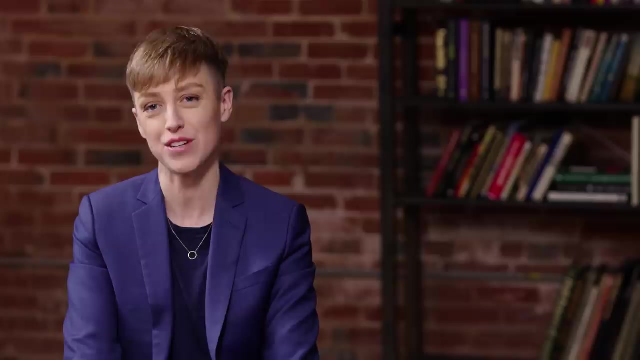 What's very surprising is the continuum hypothesis has been completely resolved, in the sense that we now know for absolutely nothing. We're absolutely certain that we will never know whether it's true or false. So this is a little bit confusing. The standard foundational axioms of mathematics that we take for granted are completely insufficient. 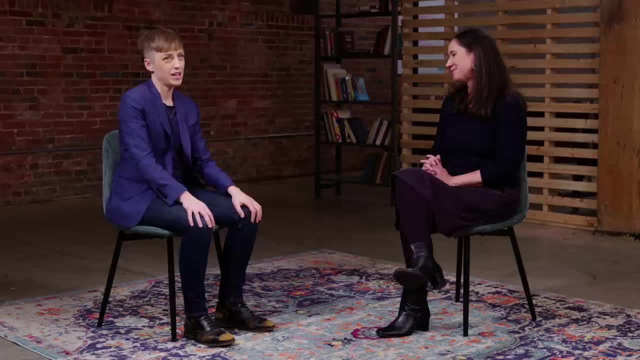 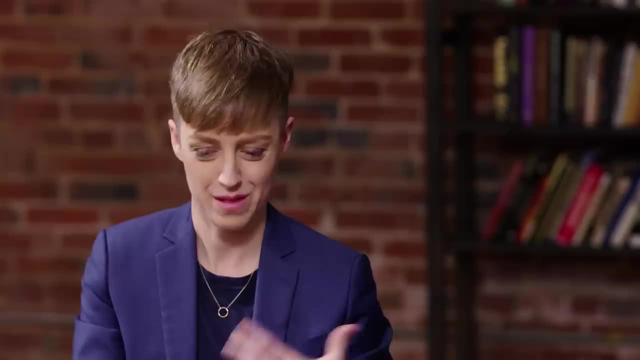 to prove the continuum hypothesis one way or the other. You know mathematicians, among other things, have been very clear about exactly what they're taking as an assumption and exactly what they're concluding from it. So mathematical practice is to be exactly transparent about the hypotheses you need. 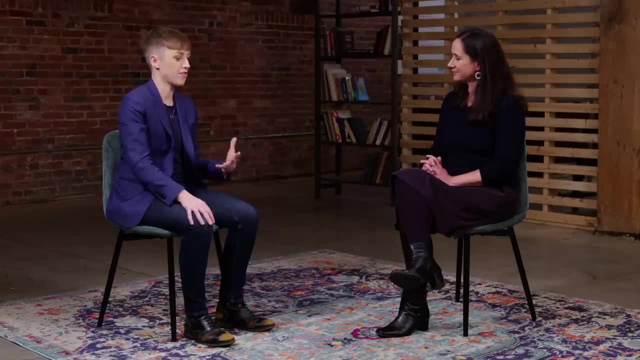 to prove your theorem. So now I think of a proof of a theorem more like constructing a function Where the domain of that function is all of the hypotheses that I'm assuming, And then the target of that function is maybe a particular element in some universe that 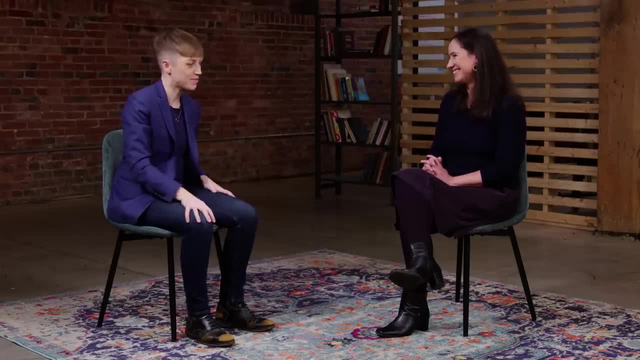 is the moduli space of the statement that I'm trying to prove, or something like this: If the foundations were to change, if set theory were replaced by something else, maybe dependent type theory, do you think the theorems you've proven would still be true? 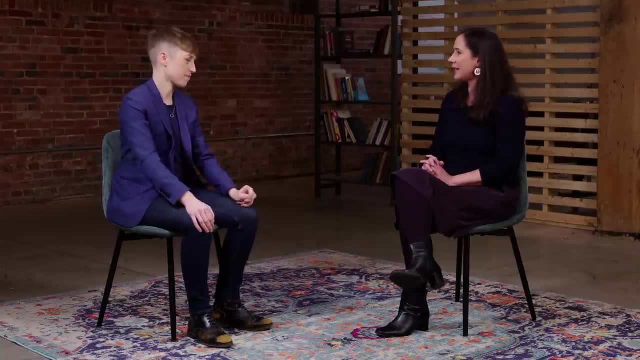 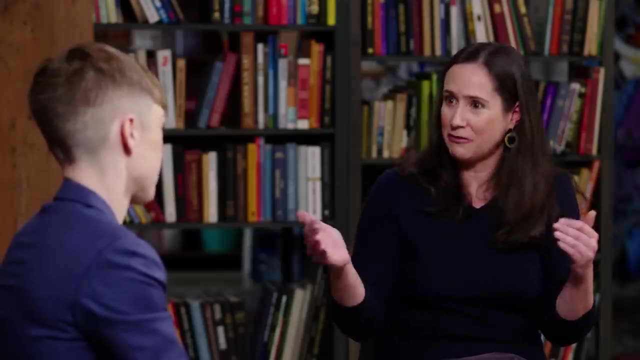 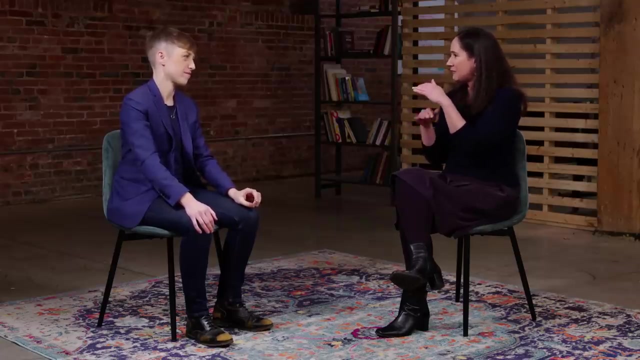 There's a lot of math that we sort of take for granted, as this is the thing that you can do. It's about really admitting that we are creating the foundations that are the basis for the work we do later, And so, yes, I think that if we change the foundations, we would change mathematics.